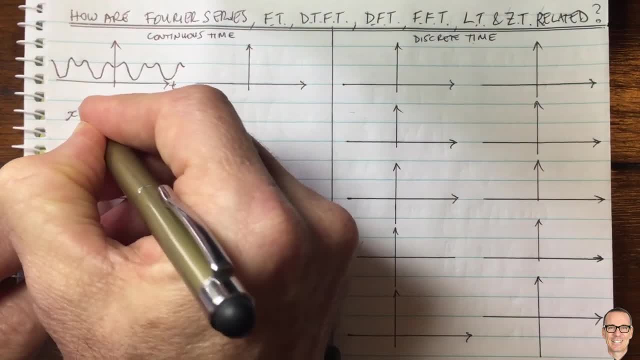 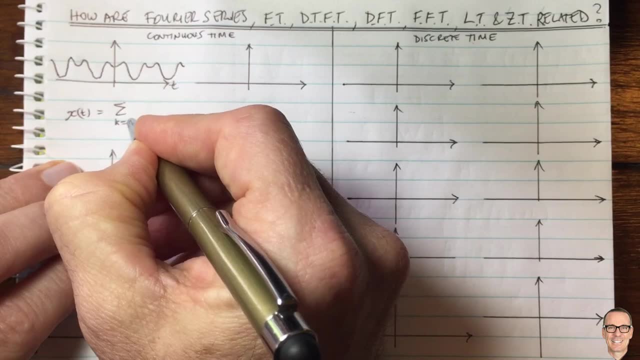 omega naught. So I'm going to write the equation here. I won't write the equation for all of the transforms, but I will for this one, just to make a point here. So this is: from k equals minus infinity to infinity of a k. 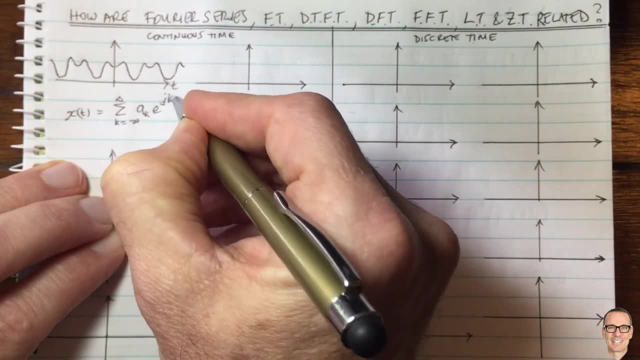 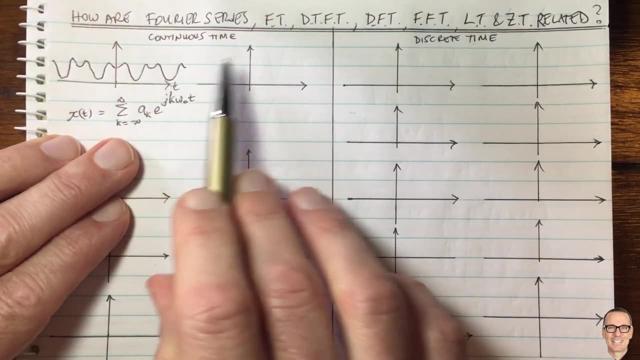 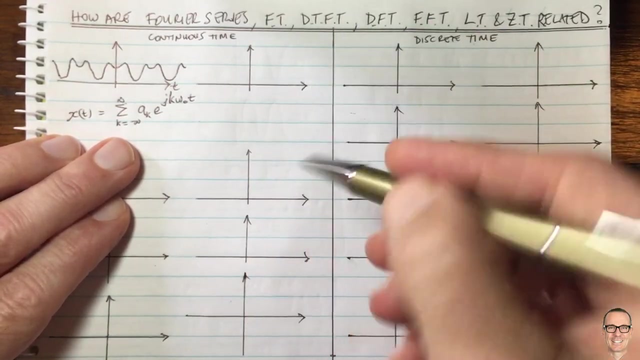 k times e to the j k, omega naught, t, And so here omega naught is the fundamental frequency. So what is the Fourier series? Well, again, I'm not going to give all of the details. There's plenty of videos on the channel. you can find in the notes below this video: 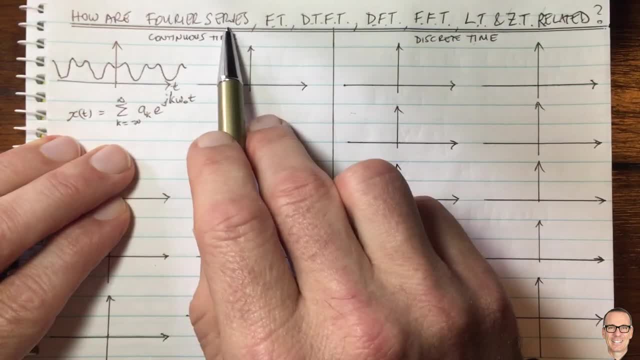 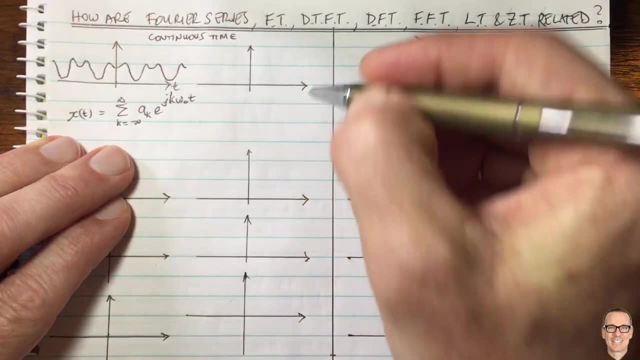 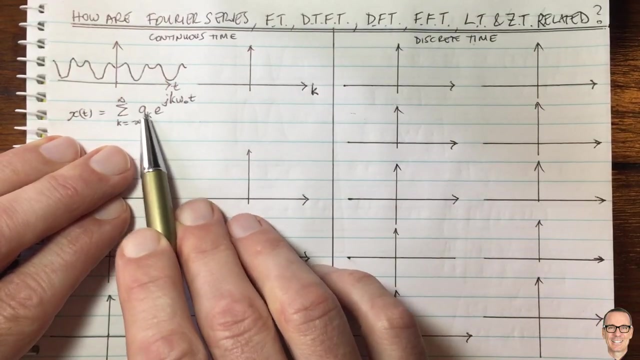 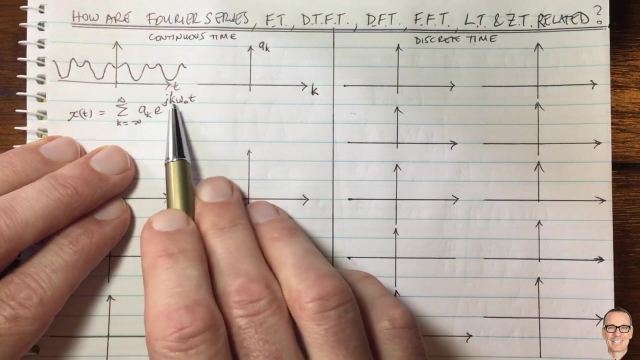 But for this continuous time Fourier series case with a periodic signal, then the Fourier series is written in terms of k. So this axis here is k, So it's not a frequency axis. This is an index of these a's. So you're plotting a k as a function of k, So it's an index of the k's and the index is related. 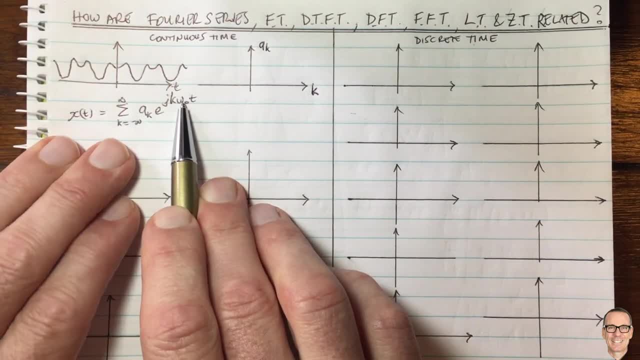 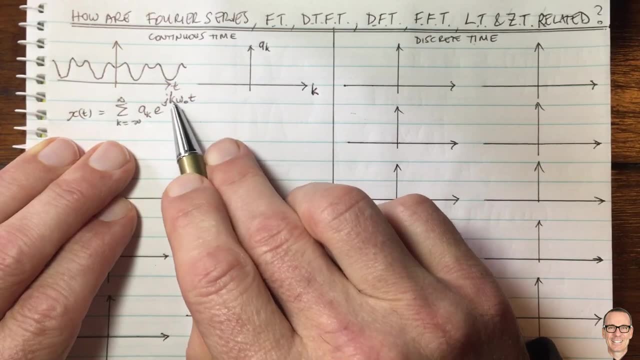 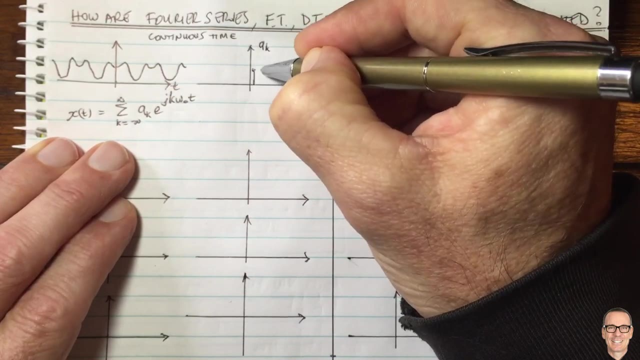 to multiples of the fundamental frequency, Okay, and in this case it is discrete because these are discrete. It's a discrete summation of multiples of the fundamental frequency components. So it's discrete and it's aperiodic. So this is not a periodic function of k, It's aperiodic. 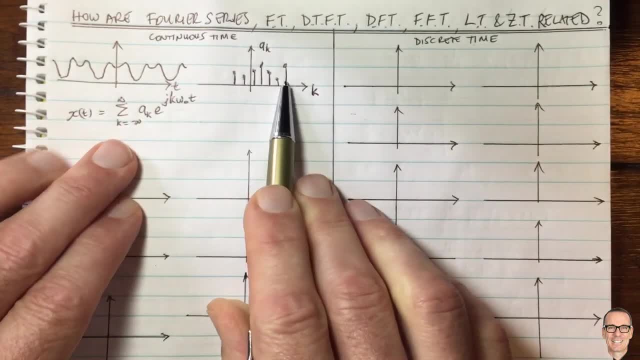 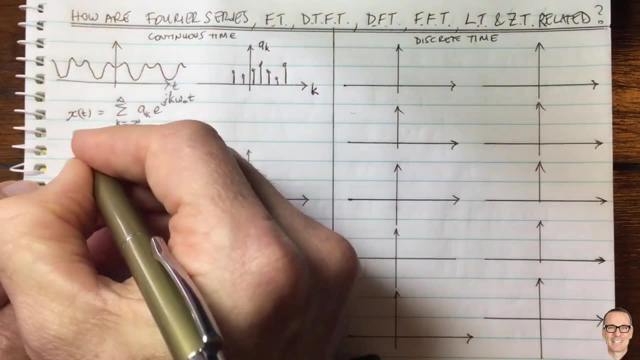 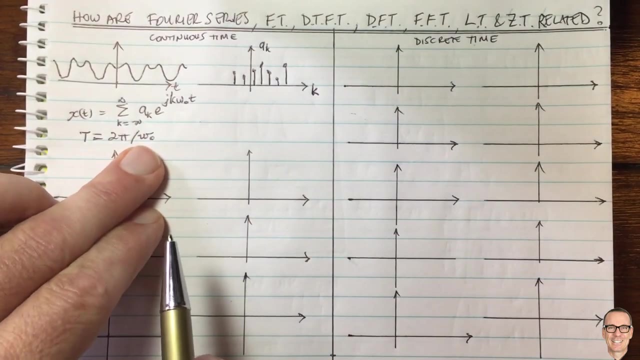 Okay, so this is one of the properties of the Fourier series. So when does it apply? Again, the important thing is it applies for periodic signals where the period here, capital t, equals 2 pi divided by that fundamental frequency, omega naught. Okay, so that's the Fourier series in. 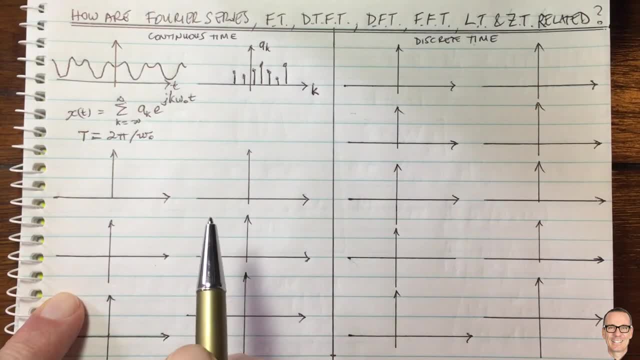 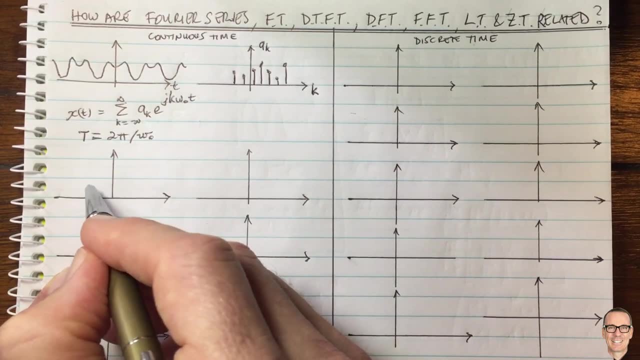 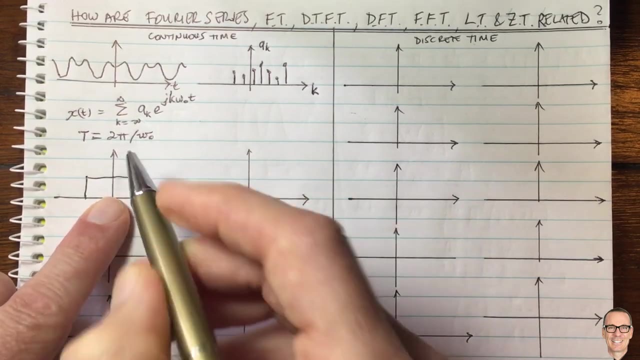 continuous time. What about the Fourier transform? Well, the Fourier transform is a generalization of the Fourier series for signals which are not periodic, And the most common signal that we, or a very common one that we consider here, is a square function. It's very important for digital. 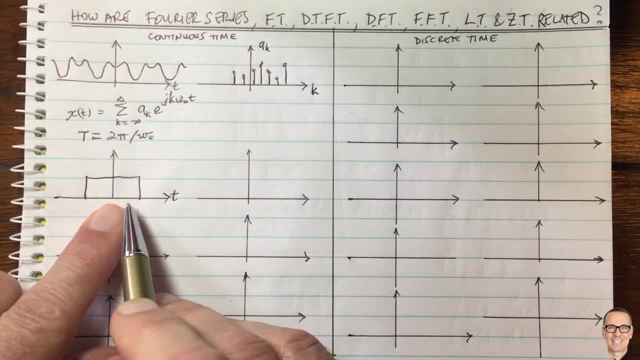 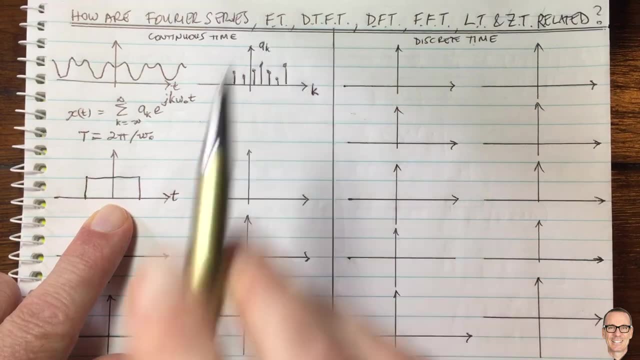 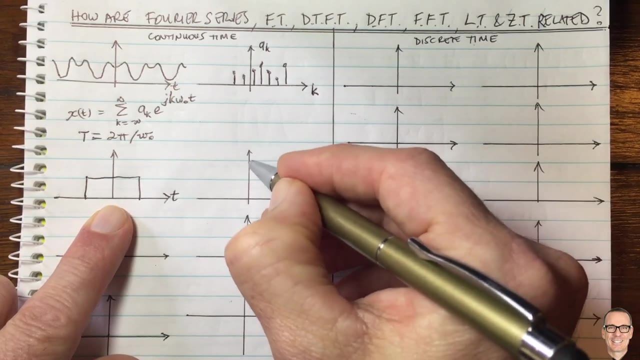 communications, where you switch something on and switch something off and all sorts of other electronics and other situations. So in this case, what is the Fourier transform? Okay, it's not periodic, and that's when the Fourier transform applies. It's more general than the Fourier series And in this case you're probably familiar with the sinc function. I'm going to be 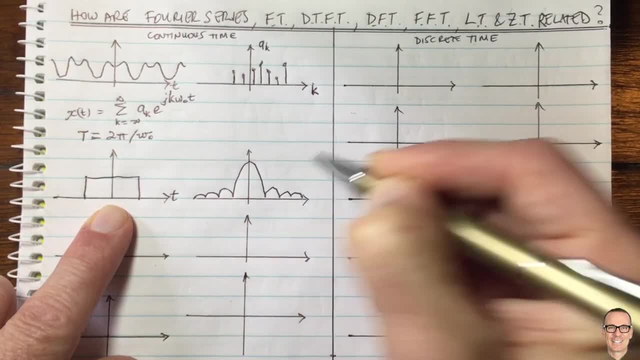 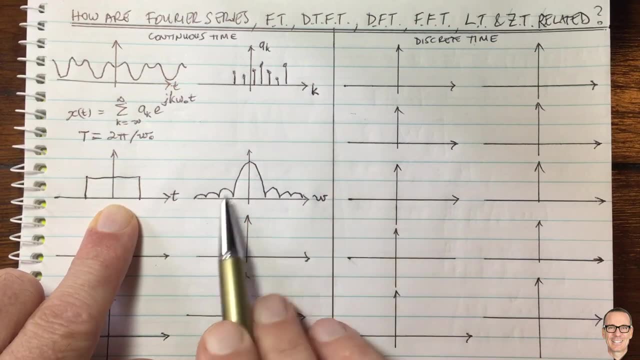 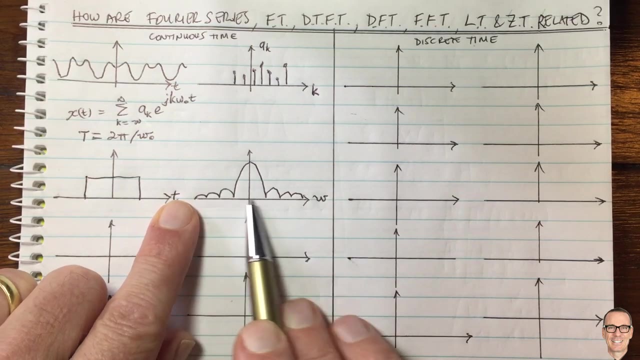 drawing here the magnitude, and this is important to remember that there is also a phase component. But in this case, some differences from the Fourier series is that this is not this. this is the actual frequency plotted in radians when you plot with omega. So this is the actual frequency and they 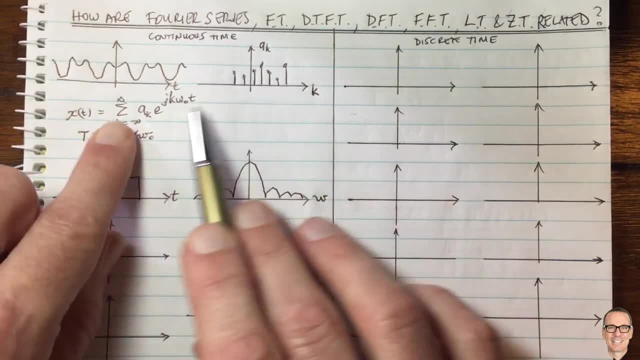 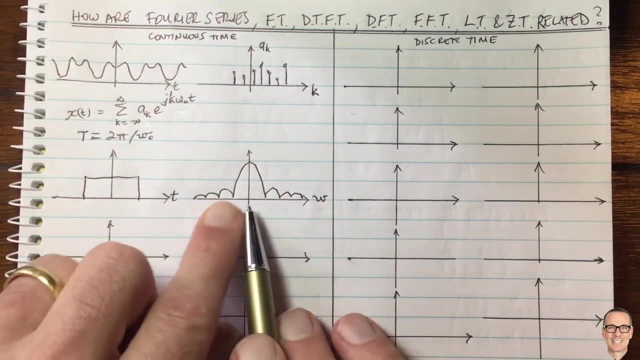 are the frequency components that are possible, Whereas for Fourier series it was only the multiples of the fundamental frequency. So that's a that's an important difference between the Fourier series and the Fourier transform. So this is all. frequencies are possible and they all can. 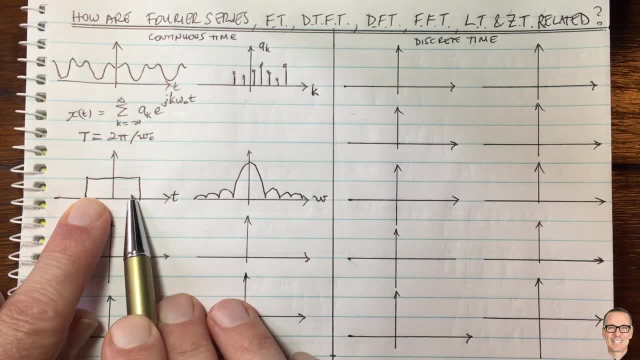 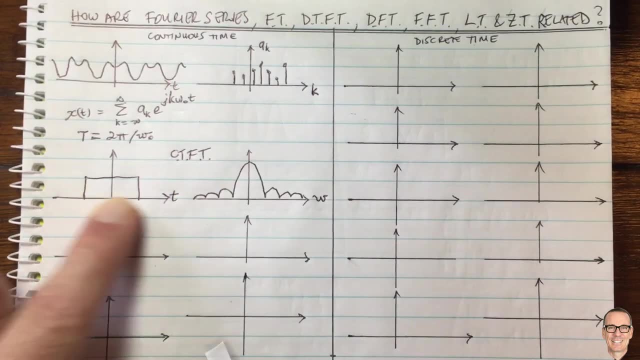 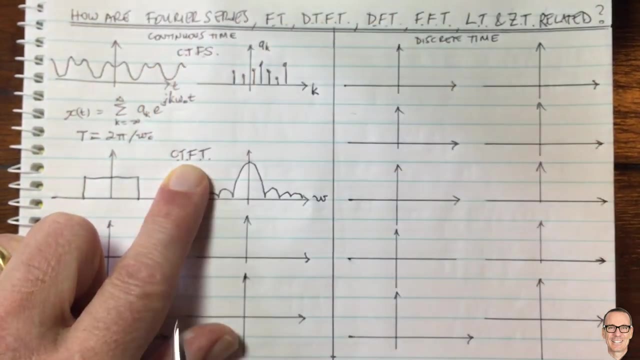 contribute to this non-periodic or aperiodic signals. So this is what we call the continuous time Fourier transform. So the c t, f, t And this one up here was the continuous time Fourier series, often c t, f, s. Okay, so this here also. it's important that I note. here I'll put a. 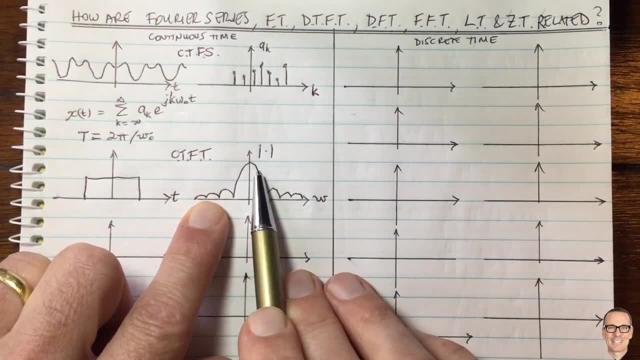 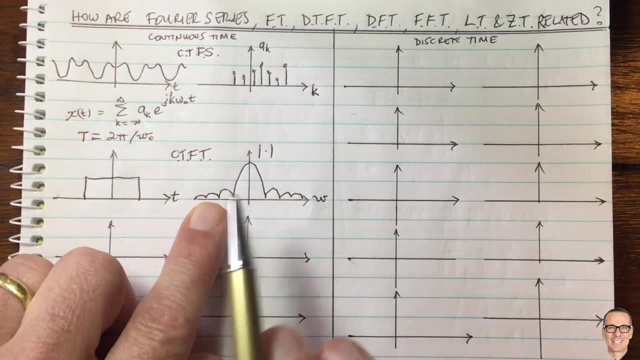 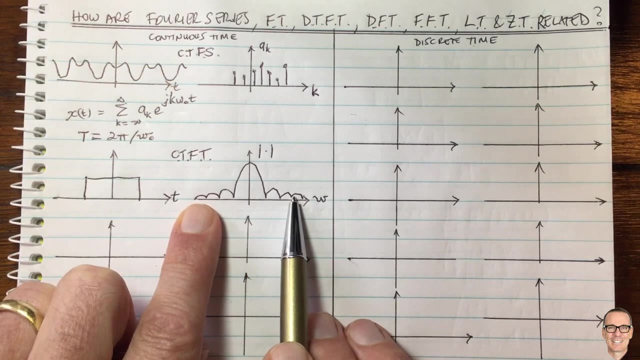 magnitude, with a dot there that there's also a phase component, but we often only plot the magnitude of the Fourier transform. So it's just something important to remember. And of course also this is continuous, as I said, with all possible frequencies, and it's aperiodic. The 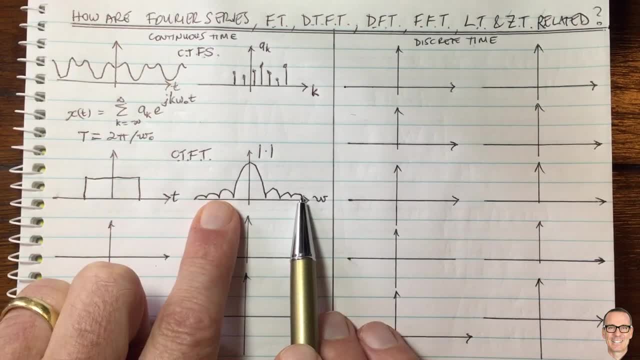 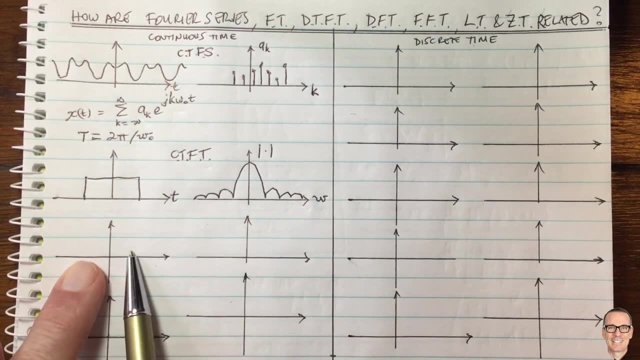 signal is aperiodic in time, and it's aperiodic in frequency. Okay, now one thing though: you can define the Fourier transform for periodic signals, And so one common one that we do is that is one of the fundamental basis functions. I'm just going to 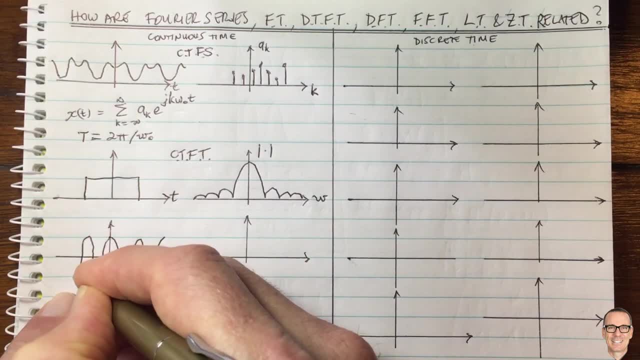 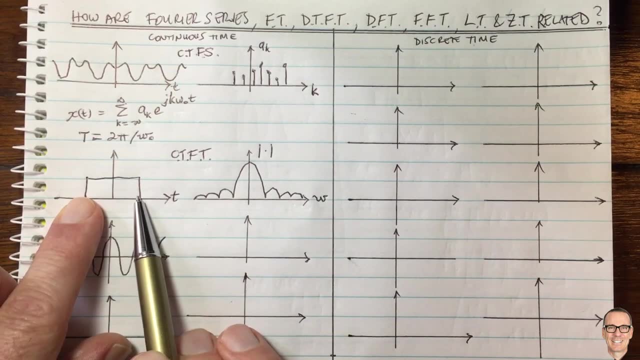 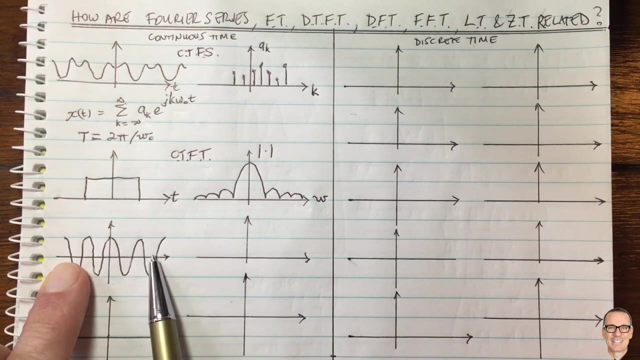 draw it here. So this is the Fourier transform for the periodic signal. So typically, one thing I should say for the Fourier transform: it's defined for signals which have finite energy. Now, these periodic signals do not have finite energy, But we can define them using the delta function. We can define them in a particular way under the 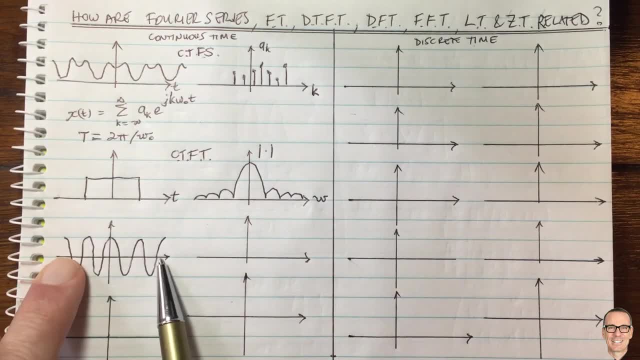 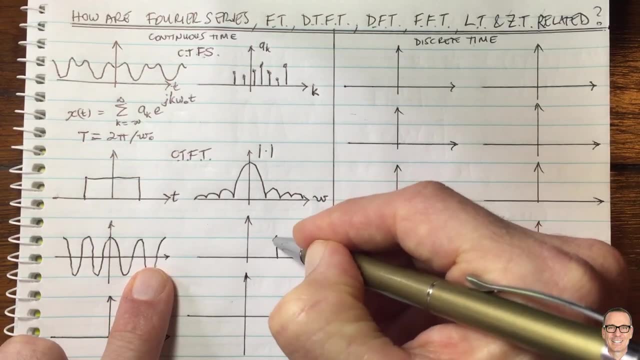 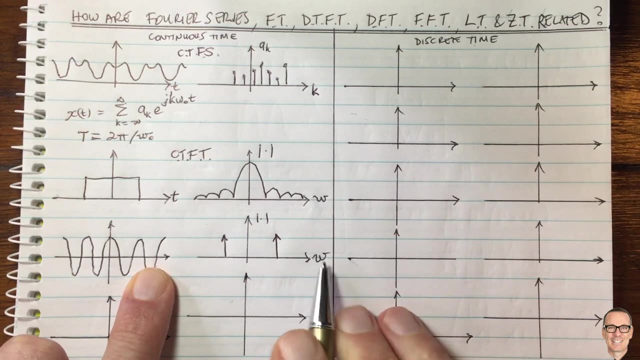 Fourier transform. So there is a definition for periodic signals under the Fourier transform And in this case for this cos wave. you might be familiar, and this is where I mentioned with the delta function, that the Fourier transform, the magnitude of the Fourier transform in the frequency domain is now actually continuous and it is impulsive. So when you have a periodic 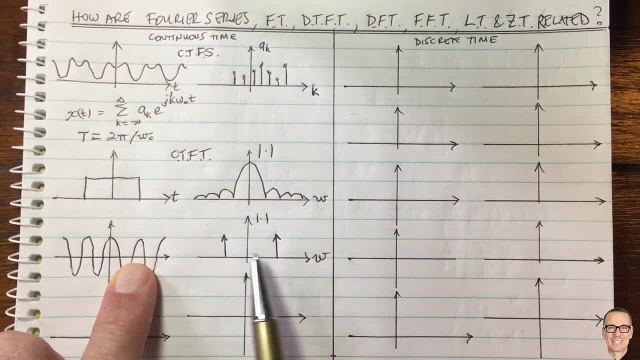 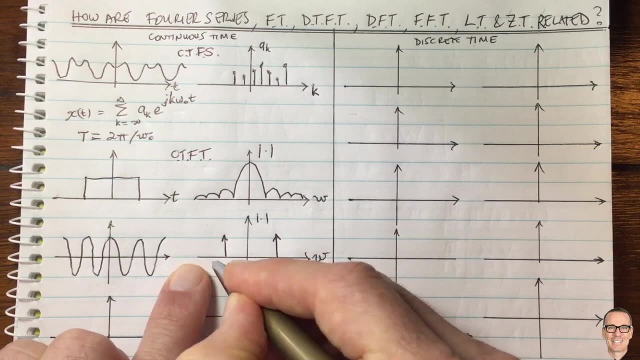 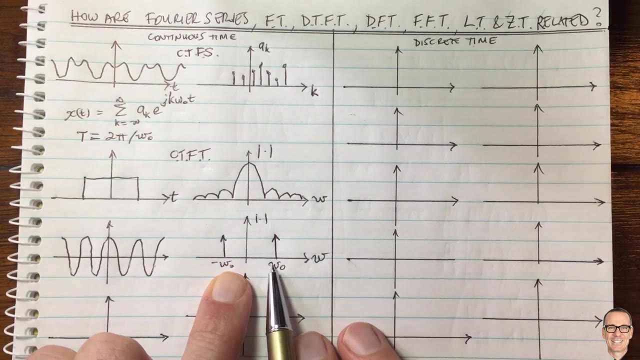 signal. if you are doing the Fourier transform, then you get an impulsive Fourier transform. We call it impulsive, where we have these delta functions And this is omega naught and minus omega naught. And again, for more information on exactly what this is, check out the videos in the link below. Okay, so 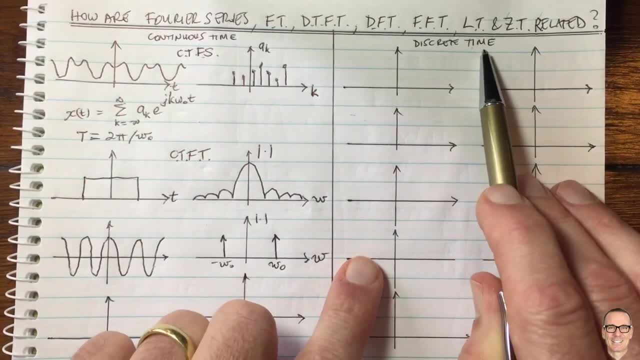 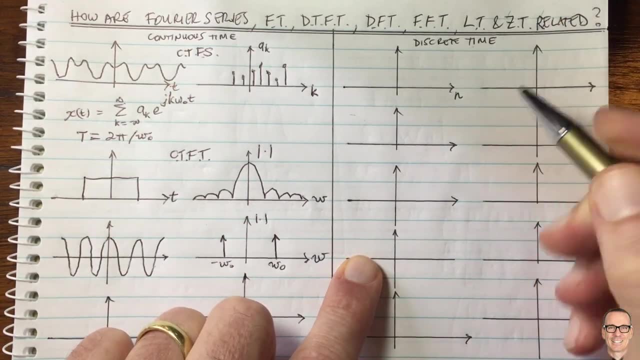 this is for the continuous time. What about for the discrete time? Well, discrete time, we have things in. we use little. typically use little things like the Fourier transform. So we have a little n to index the discrete time And we're going to start with the Fourier series in discrete 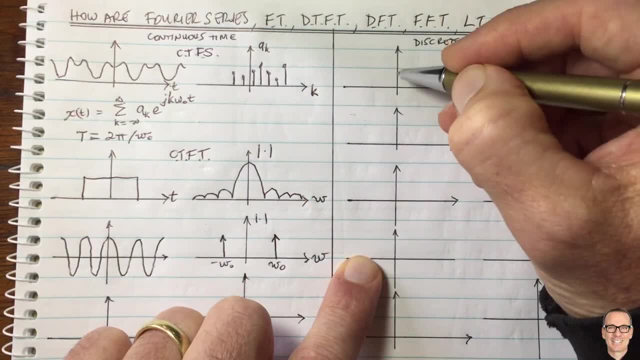 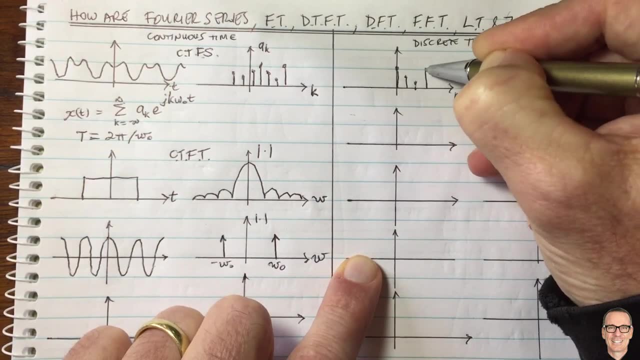 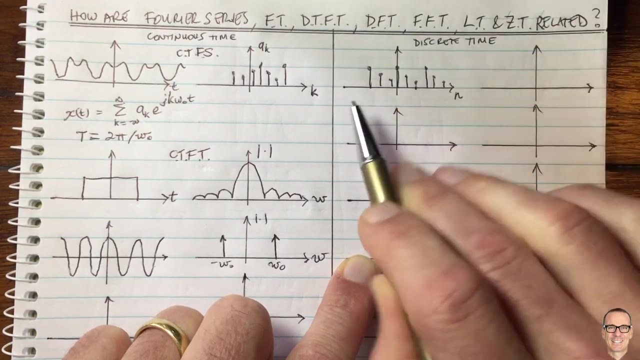 time. So again, the Fourier series relates to periodic signals. So here's a signal that is periodic. This signal here is periodic. I'll just try and sketch one here that's periodic. Okay, so this is a discrete time, So it only exists for integer values of n in the time. 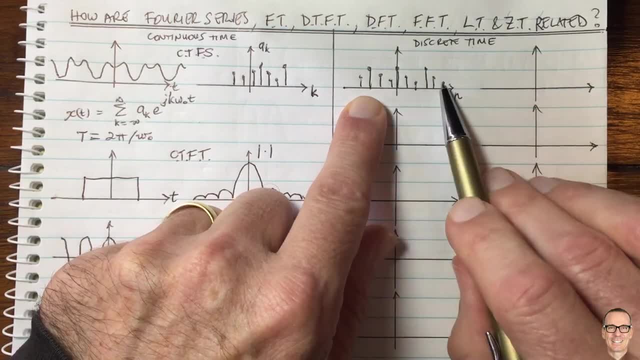 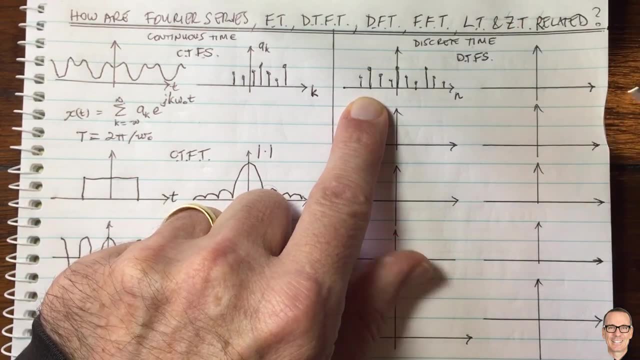 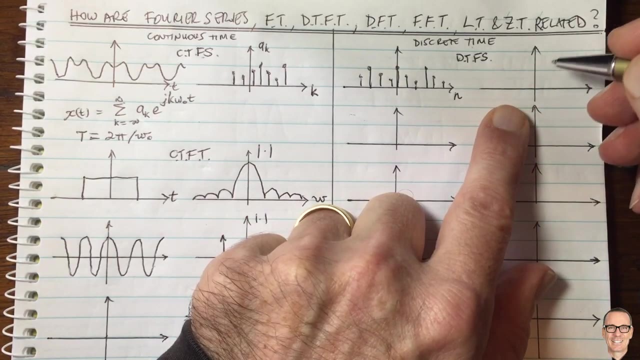 domain. So this is why it's called discrete time And it's periodic. So we're looking at the Fourier series. This is the discrete time. Fourier series DTFS. In this case it is a discrete similar to in continuous time. This time it is discrete but it is periodic. So this is turns out, this is. 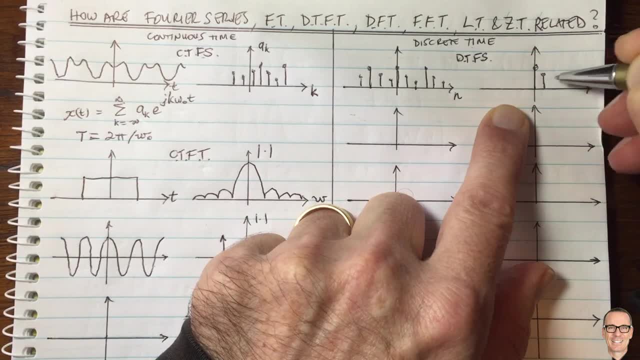 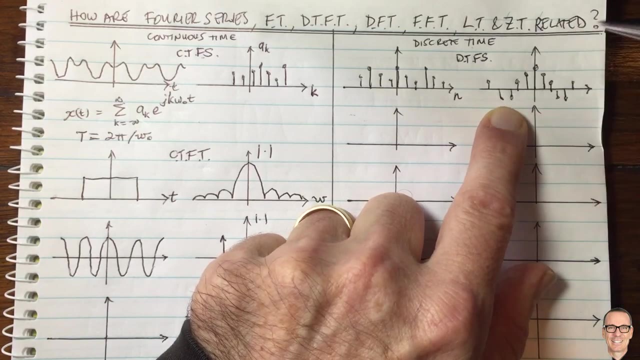 periodic. So why is it periodic? Let me just draw something here that is periodic. It's just a sketch representation. It's not exactly the. I'm not exactly trying to replicate the Fourier, Fourier series for this function over here, But I'm just trying to indicate that it is periodic. 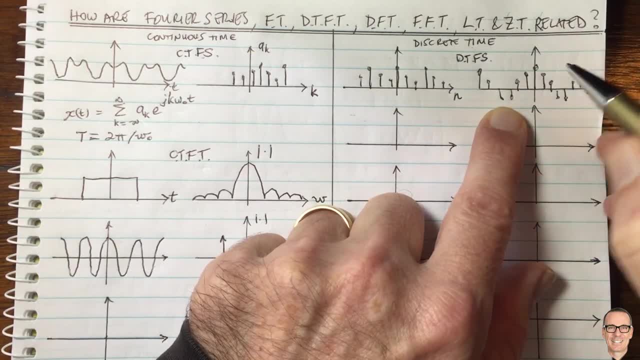 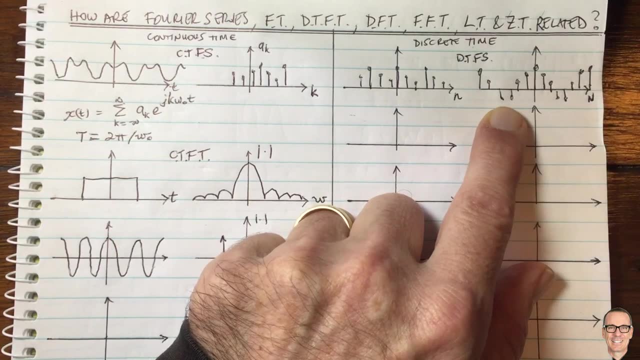 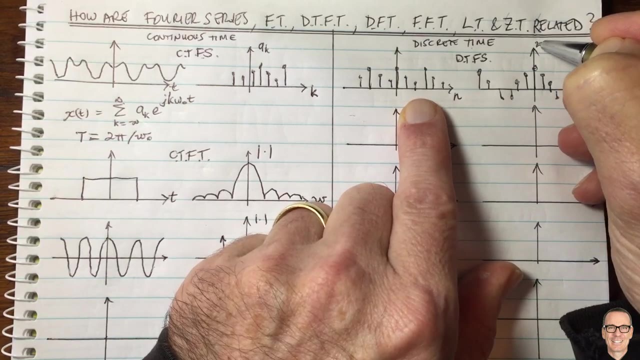 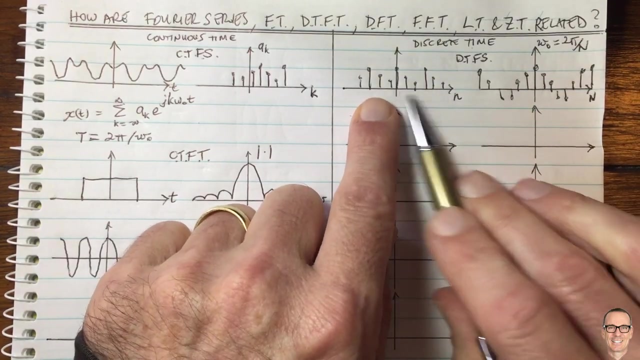 So this is a periodic function here And the period of this function is n. So this is capital n is the period of that function where you have the Fourier. the period here relates to the fundamental frequency. sorry, It relates to 2 pi divided by capital N. Okay, so this is. the period over here also is n, So this is. 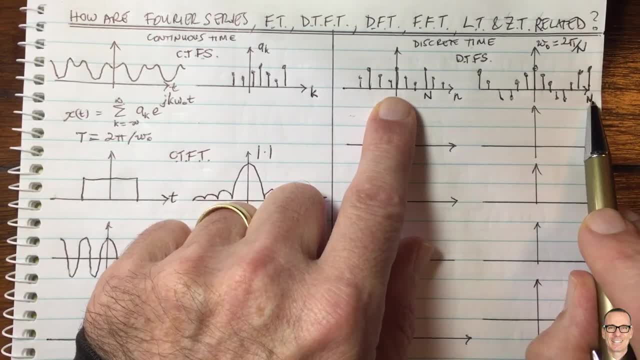 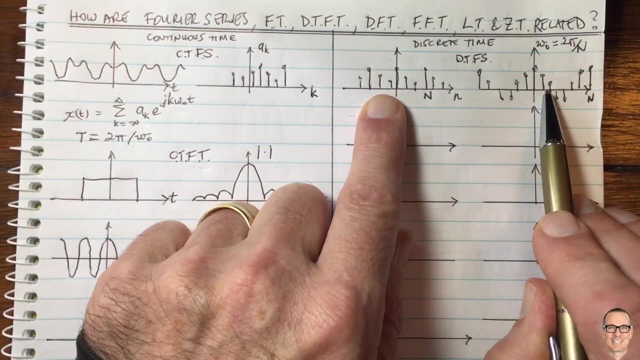 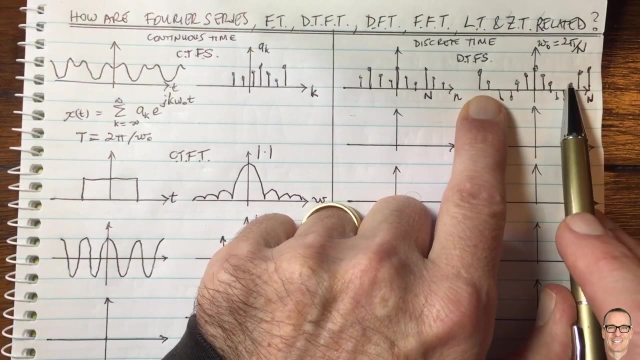 the period n- And this is in the frequency domain- also has a period n. Actually, I haven't sketched enough points in here to be exactly precise, But I think you'll get the message. So this is in the time domain, the discrete time domain, And the Fourier series is discrete and periodic, with 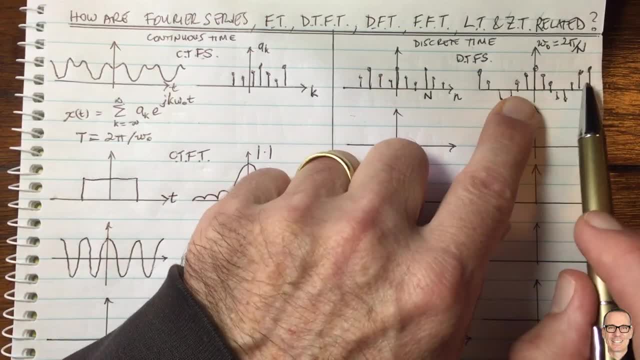 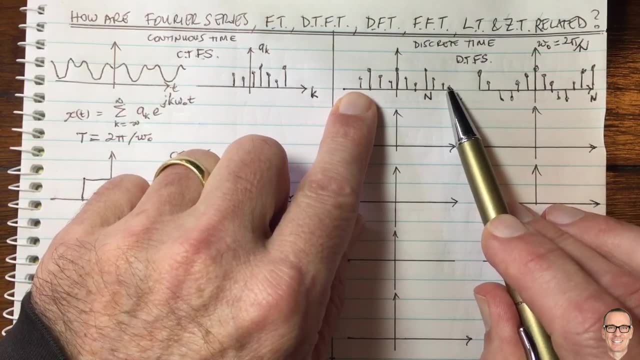 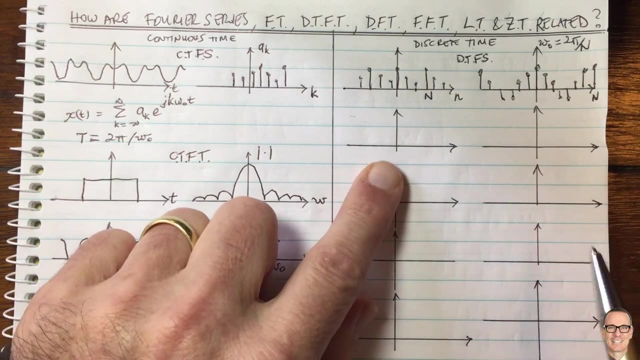 period n. So this is so one point to note. as I mentioned the, the basis functions repeat when you have discrete time signals, And so for more information on why they repeat it's, there's plenty of links in the description below where you'll be able to find information on that. Okay, so now let's look at the. 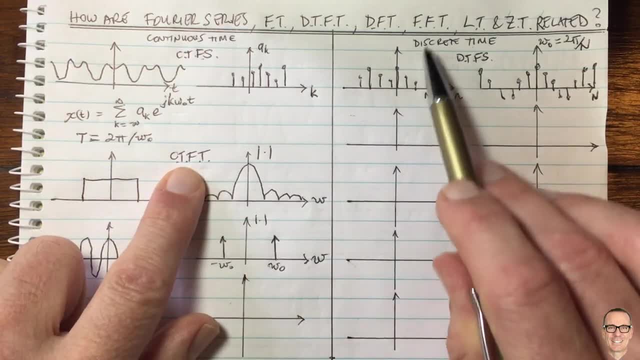 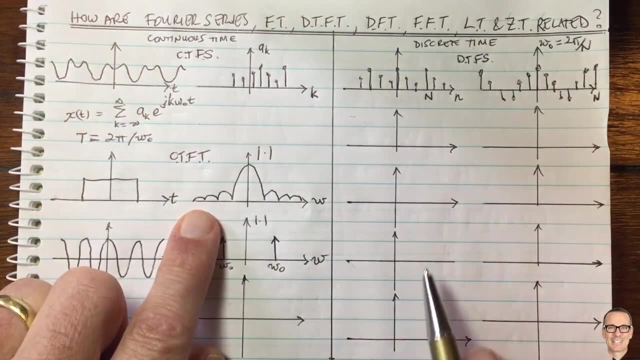 equivalent to this one over here. So now we've got the Fourier transform in discrete time. So what do we look at here in a common one equivalent to this one over here? I'm just drawing it with an offset here because I've got a square. 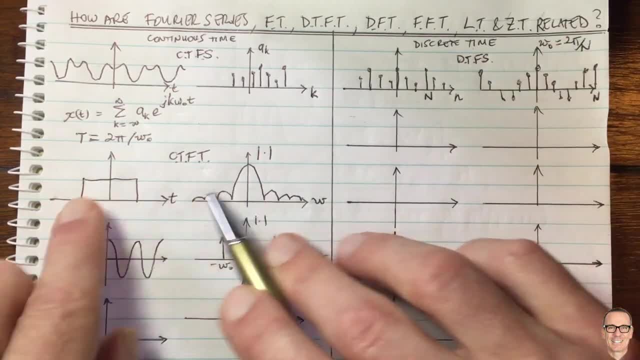 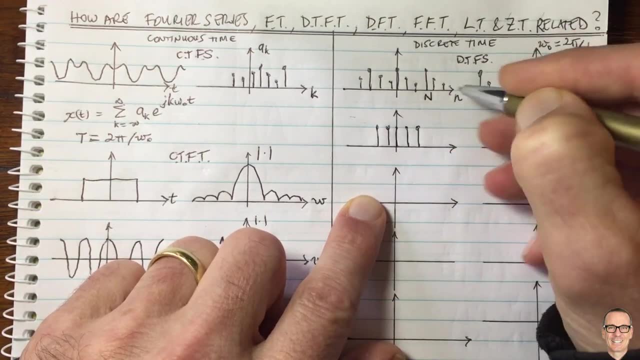 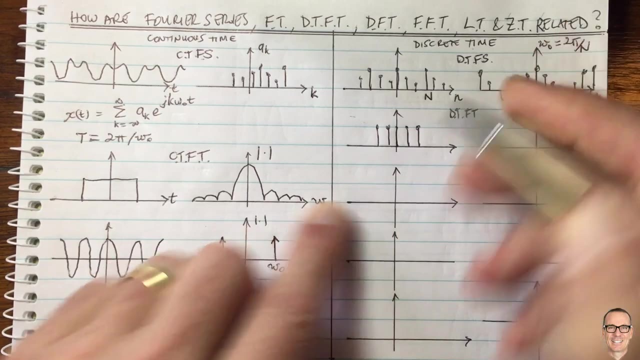 So we can squeeze one more in on the discrete side. So hopefully you recognize that this one is going to be equivalent and matching up to this one over here in terms of that. this is the discrete- sorry, the discrete- time. Fourier transform. So this is the transform line and this is the transform line on discrete time. 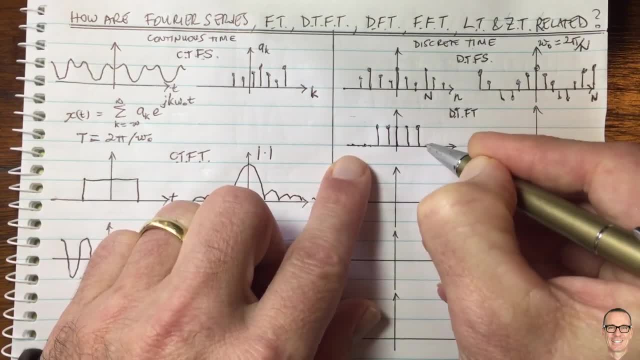 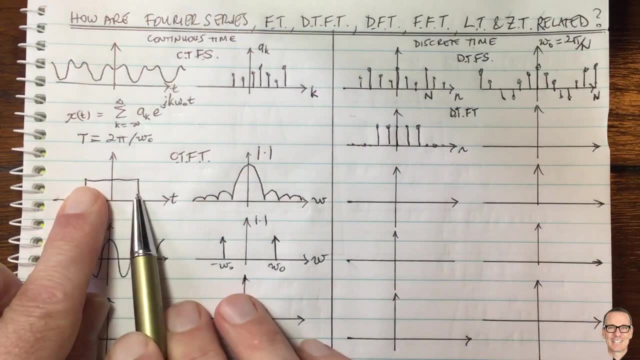 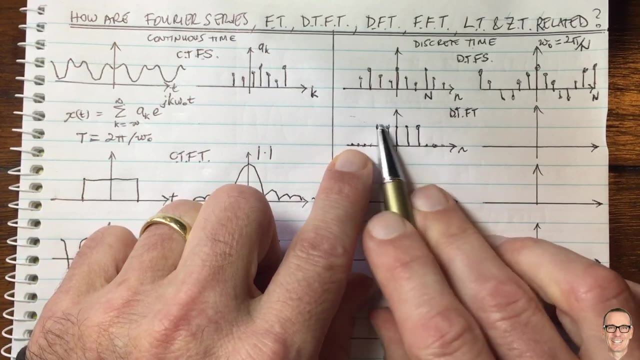 So here we've got. it's important not to forget these zeros off here. So in this case here, this function here is aperiodic. Therefore we need the Fourier transform, just like we had in continuous time, and it's zero for all the different times other than these times here I'm just using this square function as an example. 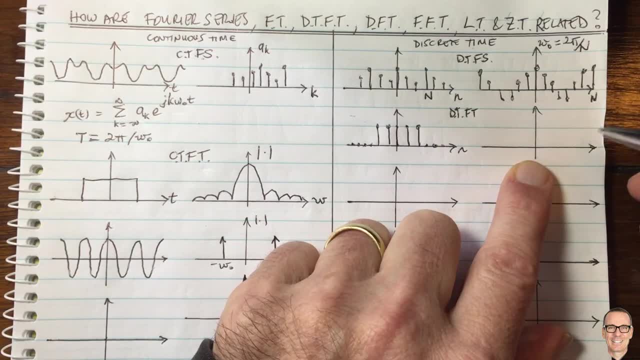 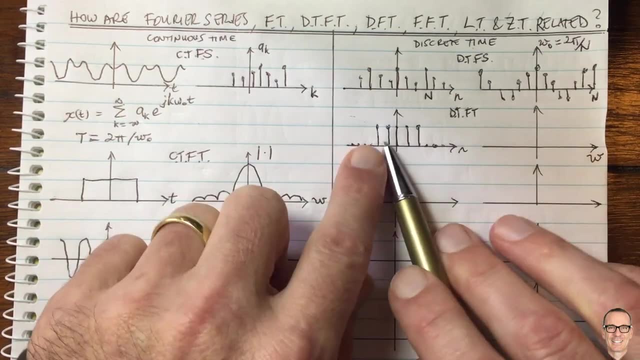 In this case, again, the basis functions repeat. What does this mean? Well, I'll draw that just in a minute, but I'll make the point first of all that the Fourier transform of a discrete time signal, that's aperiodic, is a continuous function. And so here's. 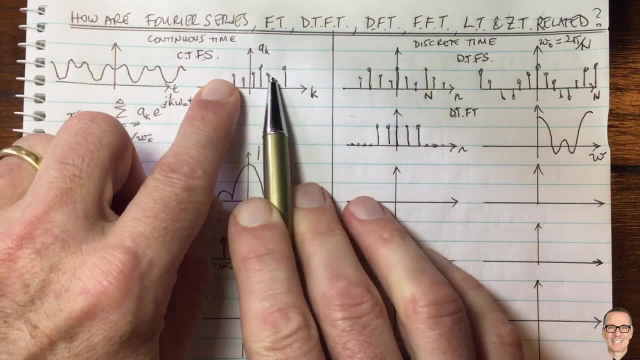 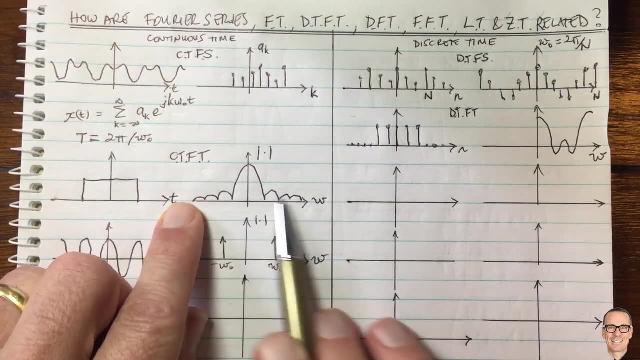 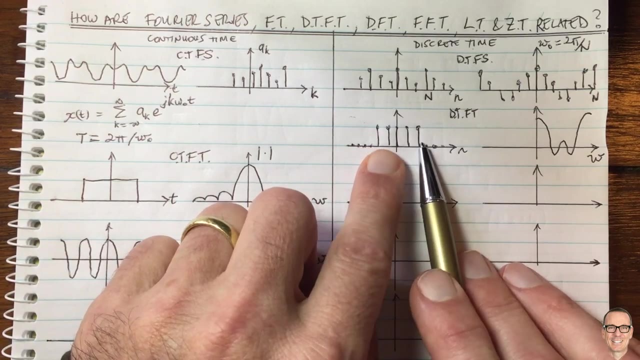 continuous and exactly the same reason for over here. This one was discrete in terms of the Fourier series, and then the Fourier transform was continuous. It had the possibility to contain all different basis functions at all different frequencies, And this is exactly the same in the discrete time case. 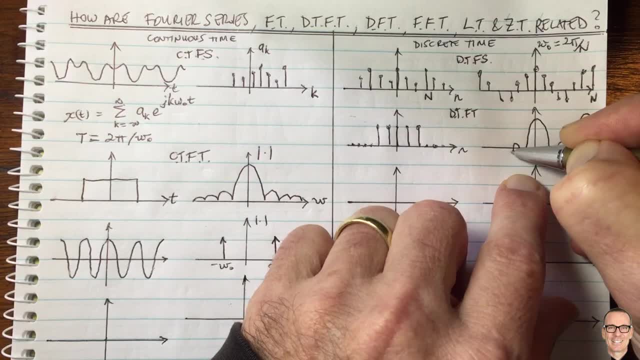 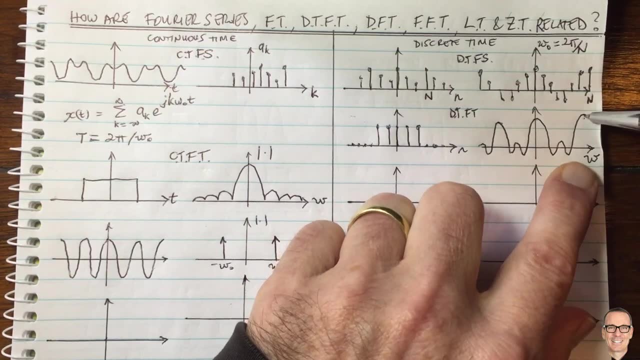 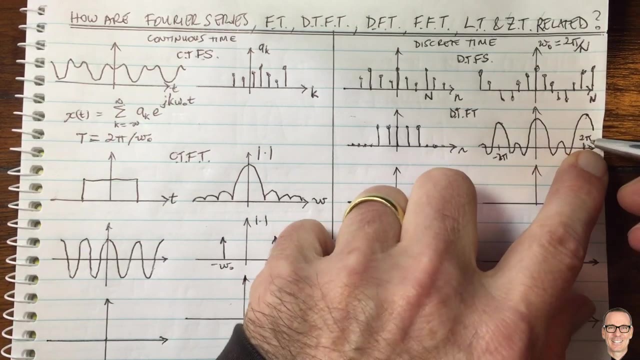 And, once again, if that's something that you would like to know more about, there's a video in the link in the description below, And so this is because the basis functions- repeat, this is a discrete function- is periodic and the period is 2 pi. so this is minus 2 pi and this is 2 pi and this is 0 here. 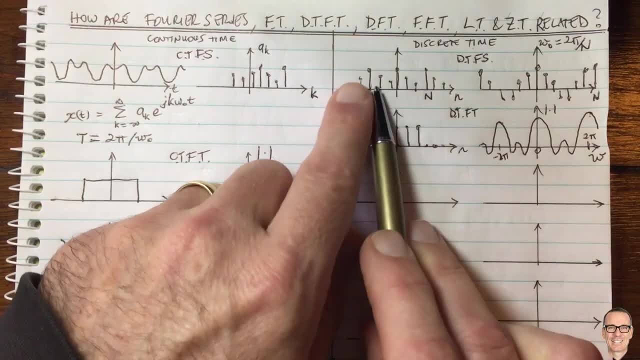 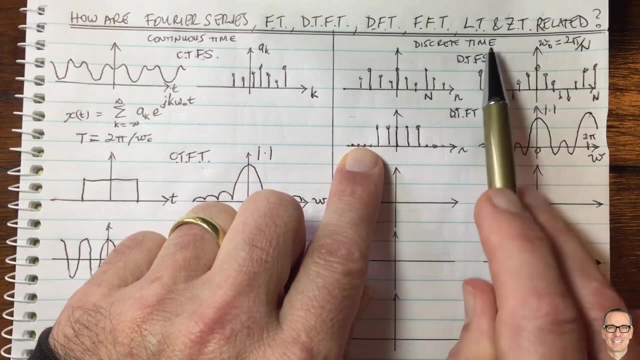 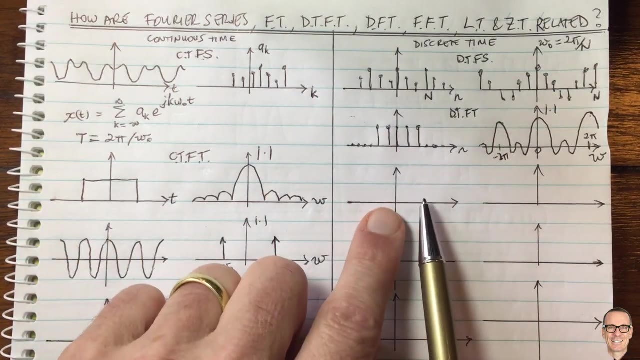 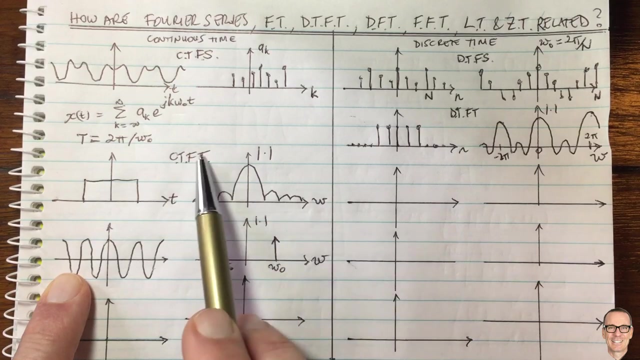 and again we're plotting the magnitude. so this is the Fourier series has discrete, is discrete in the Fourier series, the Fourier transform. even though it's discrete time, the Fourier transform is continuous. okay, so we've got aperiodic signals. now what about the periodic signal in discrete time to match with this one over here? so we said the Fourier transform was for. 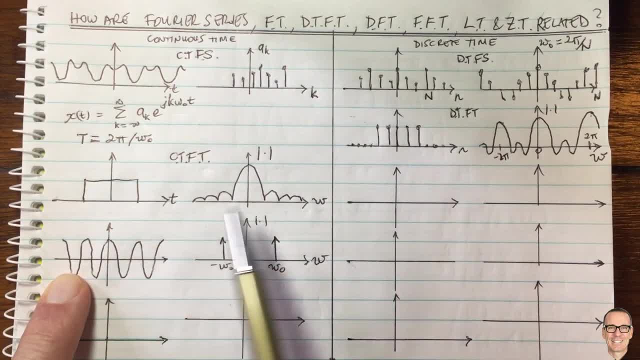 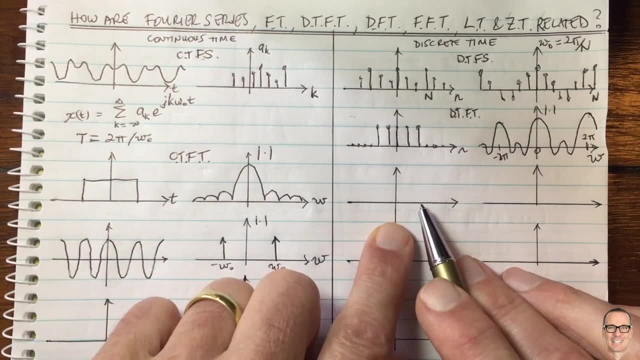 aperiodic signals, signals that are not periodic, but you can define it as the same in continuous time. you can define the Fourier transform in discrete time for a periodic signal. so let's pick one here, for an example. let's pick the matching this one over here. 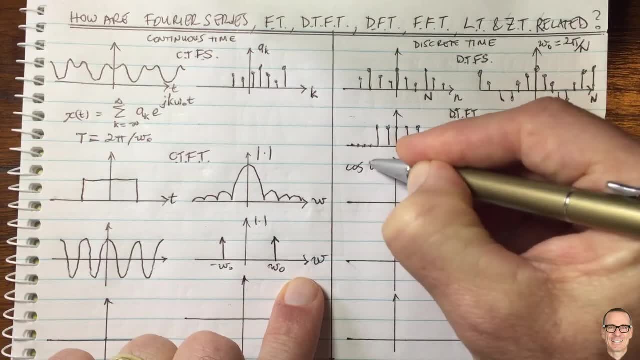 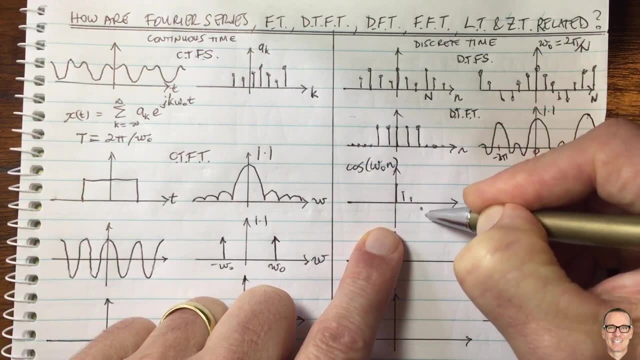 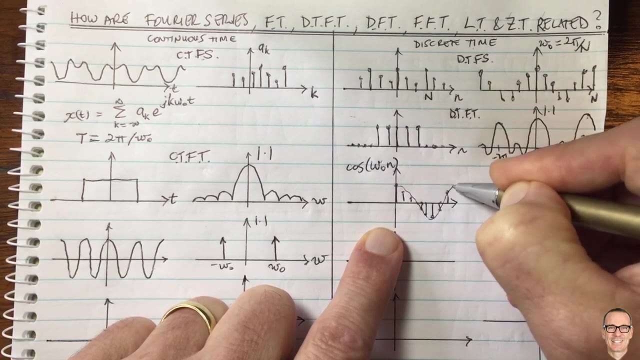 so let's pick cos omega naught n. so this function here, cos omega naught n looks like this function here. it, where it goes, sort of follows a cos shape. so I'm just drawing the that curve. there is an indicator of where the points are. I'm not trying to fill it in, just 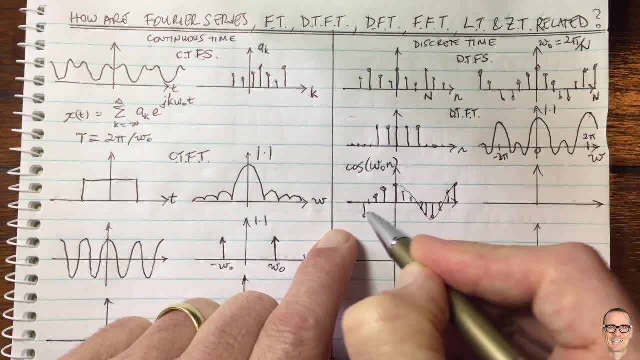 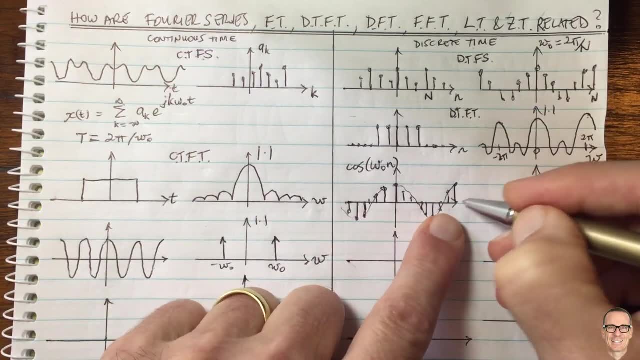 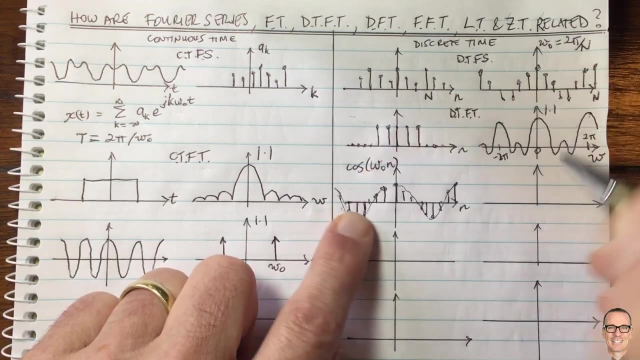 these are the actual discrete points here of a cos function in discrete time. okay, so this is a just trying to sketch that in there. so this is in discrete time. a periodic function can have a Fourier transform, so let's remind ourselves. it's in this case because it is a 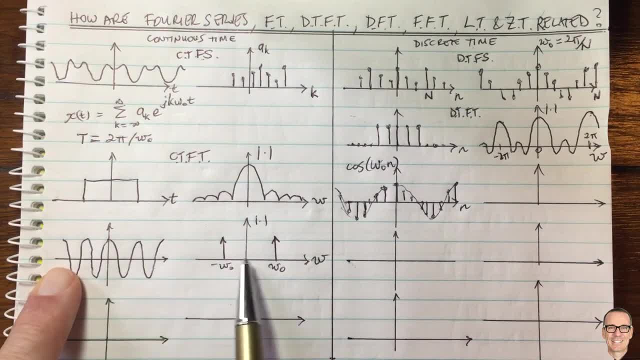 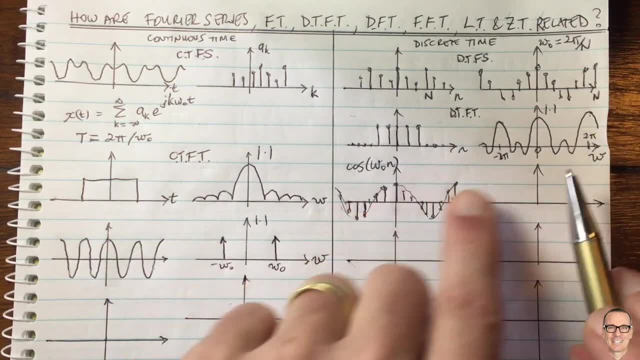 periodic function. just like in this case, over here, the Fourier transform is going to be impulsive. so over here, in discrete time, the Fourier transform of a discrete time signal is still continuous. so it has potential to have a Fourier transform, but it's not going to be. 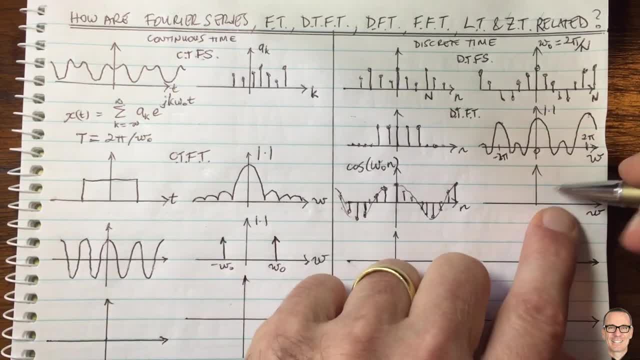 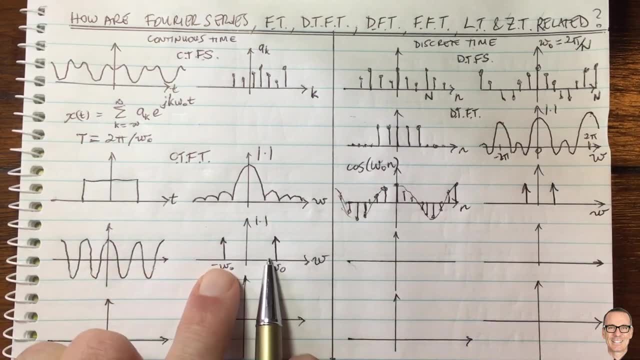 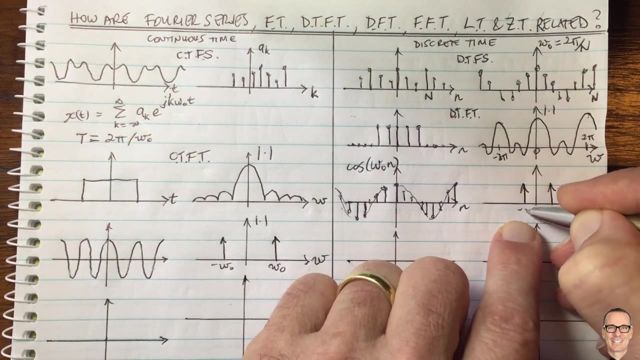 all the values of omega. but because it is periodic, this is going to be impulsive, and so here, for example, we're going to have matching with the continuous time version. we're going to have these two impulse functions at omega naught and minus omega naught, but again because the basis functions. 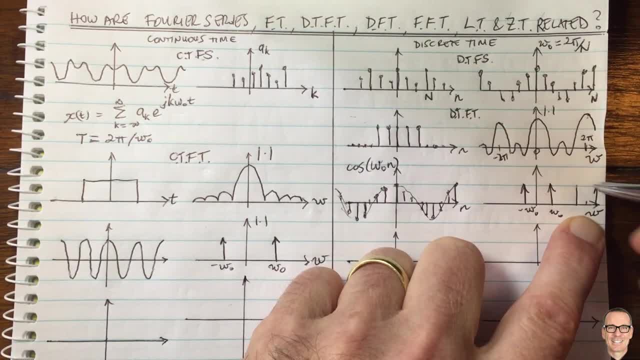 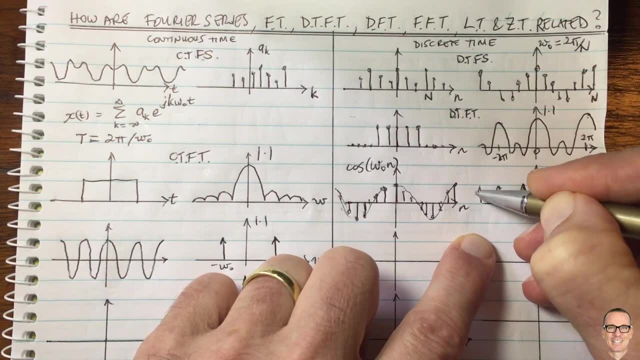 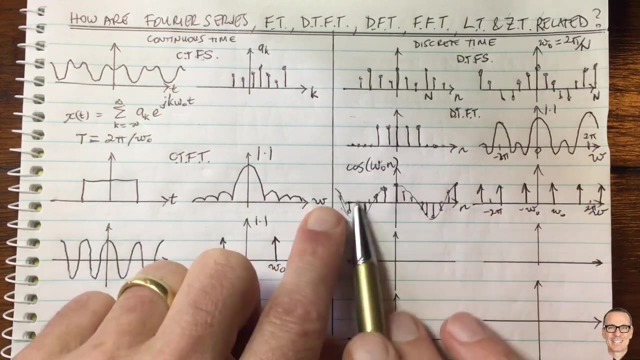 repeat. we're also going to have those repeating around centered at 2 pi and also repeating centered around minus omega naught. so we're going to have these two impulse functions at omega naught minus 2 pi. so this is minus 2 pi, this is 2 pi and this is the Fourier transform of a periodic. 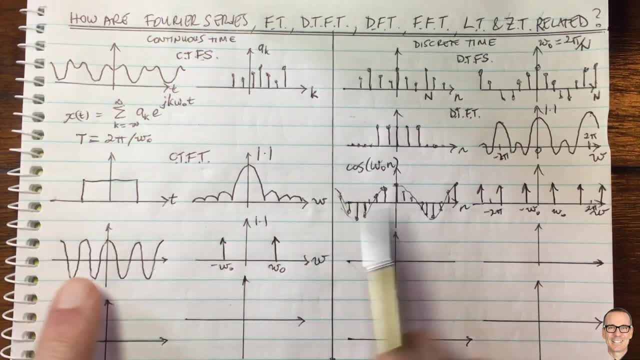 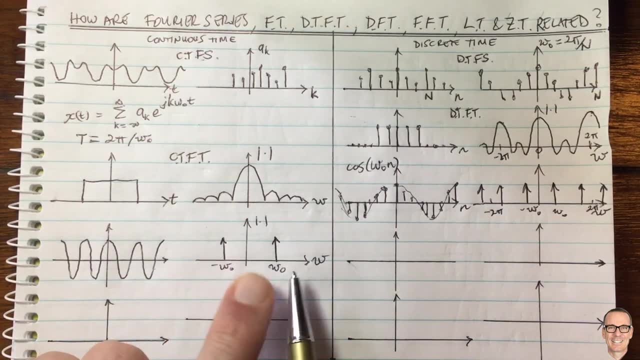 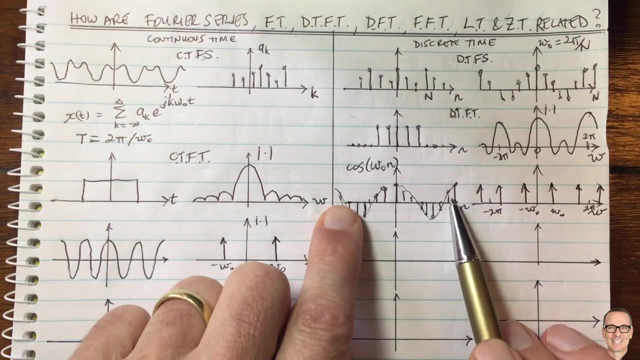 discrete time signal so it matches. you can look at the the similarities over here. in continuous time, the continuous time cos waveform has a Fourier transform that just has two impulses at minus omega naught and omega naught. in discrete time it also has two impulses, but because it's in discrete time the basis functions repeat at 2 pi and multiples. 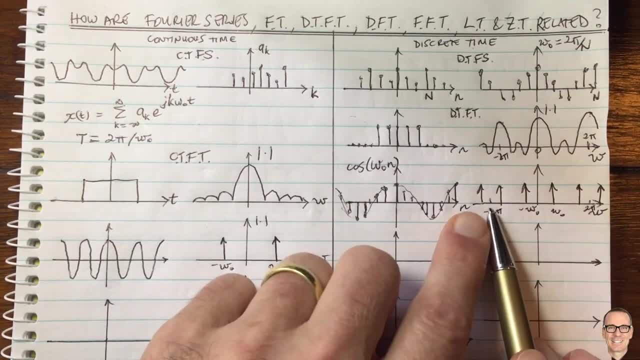 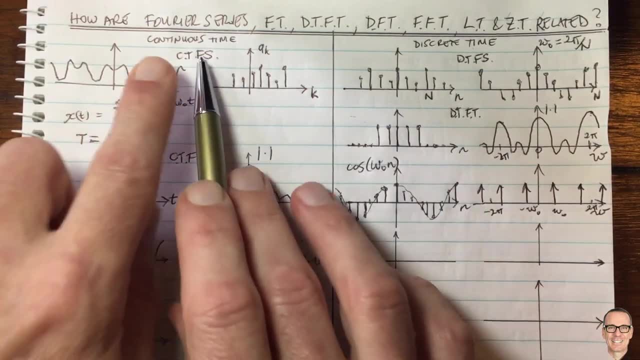 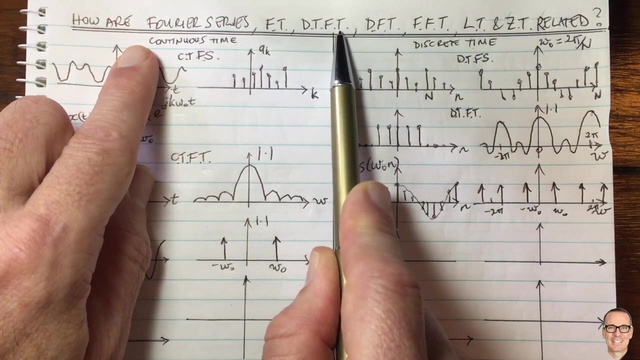 4 pi, 6 pi, 8 pi and so on, as well as minus 2 pi, minus 4 pi and so on. so this is the, the equivalence across from continuous time to discrete time. okay, so now we've covered Fourier series and Fourier transform and the discrete time, Fourier transform. so what's this other thing called the? 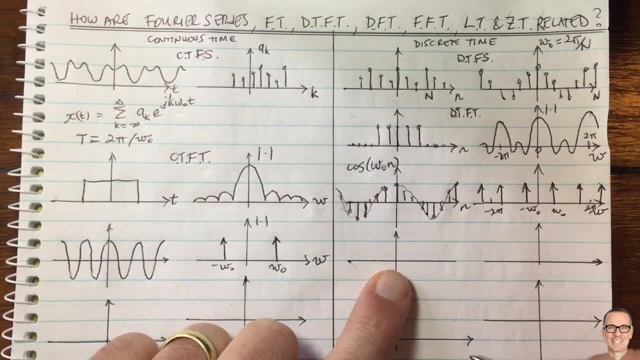 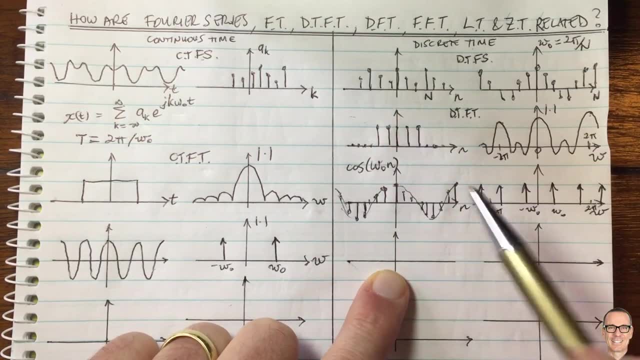 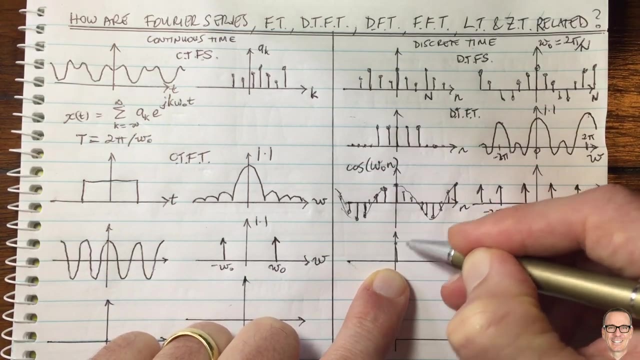 discrete Fourier transform. well, the discrete Fourier transform is mostly what you implement in a computer, and this is because a discrete Fourier transform is a discrete Fourier transform, is just an equivalent of the discrete time Fourier transform, but where you only have a finite number of samples. so in this case here, because this is what you've stored and you've measured- 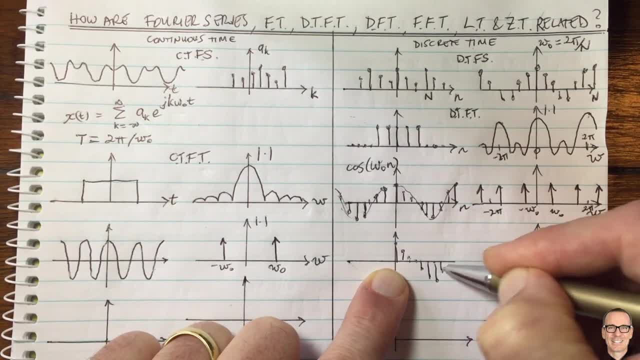 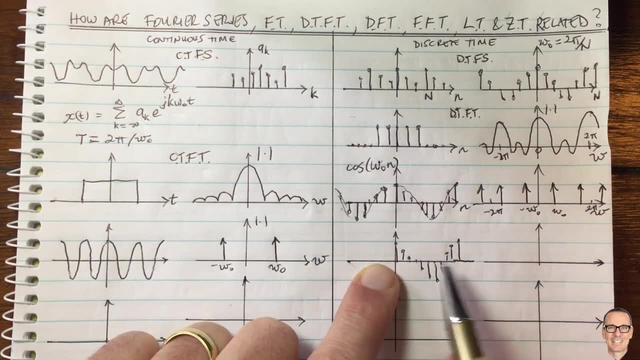 and you've stored on a computer. of course, in reality you don't have an infinite number of samples, so you only ever have a finite number in reality. and so if you've sampled, so what does the discrete Fourier transform? so this is the DFT. what does the discrete Fourier transform do? is you? 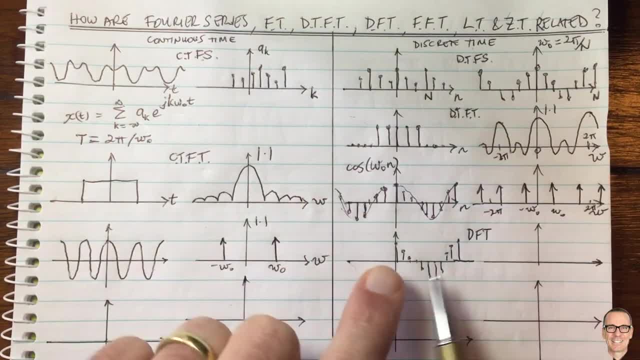 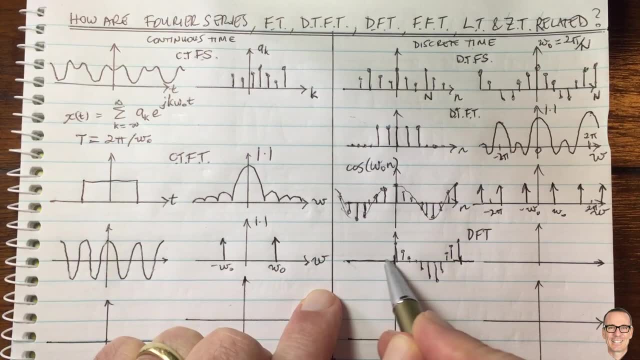 have a finite number of samples. so this is the DFT. what does the discrete Fourier transform do, is you? what's the difference between this and the discrete time Fourier transform? well, as I say, it only knows about the samples between two limits, so it doesn't know anything about the samples out. 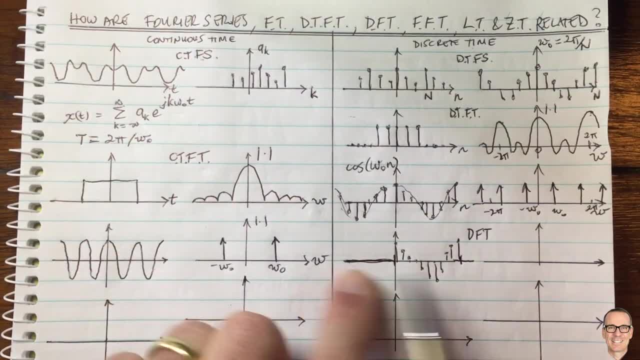 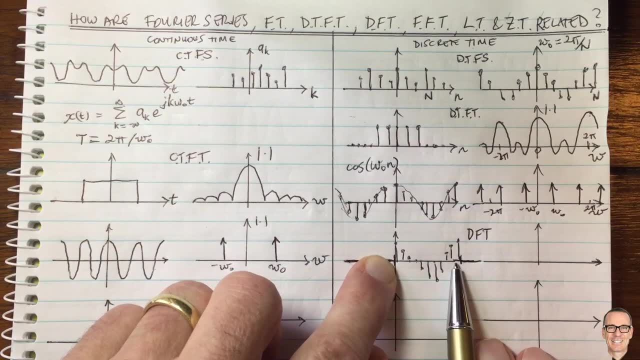 here. it's not that they're zero like they were out here, they just don't exist. all you've done is sampled for a finite amount of time, so you've got a finite number of samples. so there's no arrow on here. it's not in n index that goes on to infinity or anything, it's just over the finite. 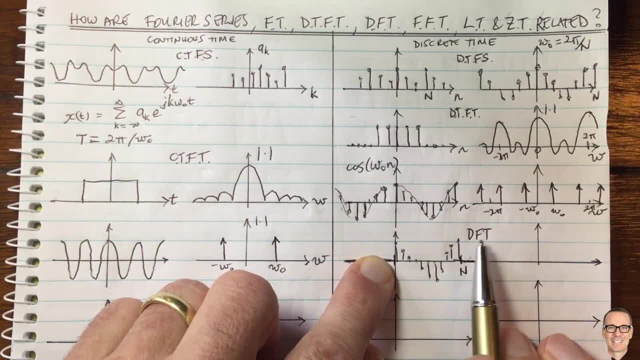 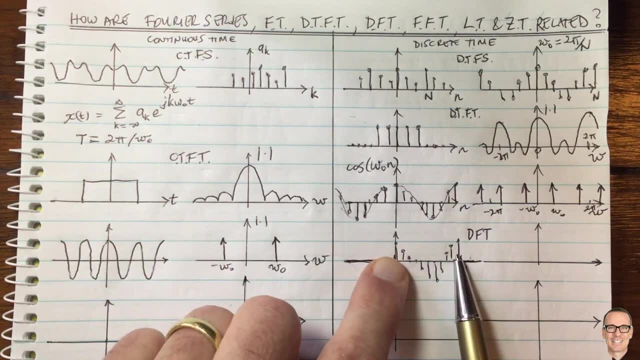 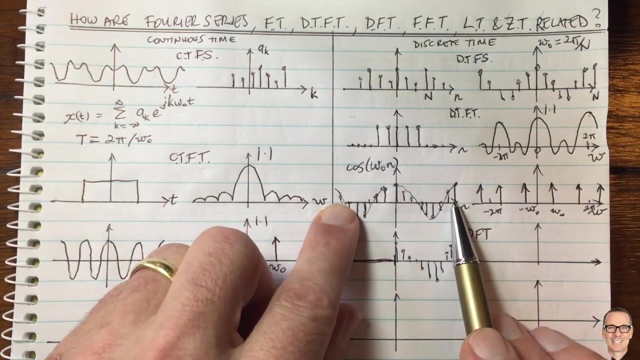 sampling period of capital N. and what does the DFT do? well, it assumes that what you have sampled is periodic. so it assumes that these samples repeat as if they were like in the example above here, as if they were a full periodic waveform that does go from minus infinity to infinity. 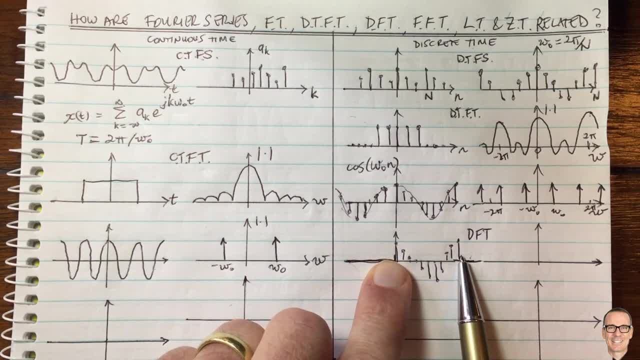 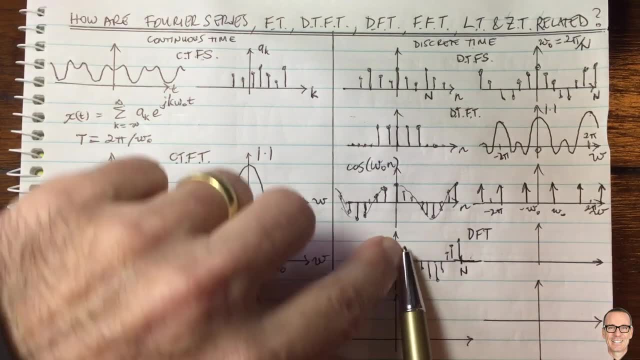 all you've done is sampled a finite number of samples, which is all you can ever do in practice. but the DFT assumes- implicitly assumes- that you have a finite number of samples, so you've got a, that you have sampled a full period from something which is periodic and does go on. 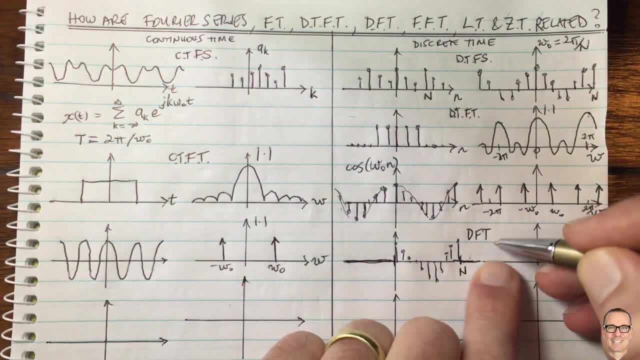 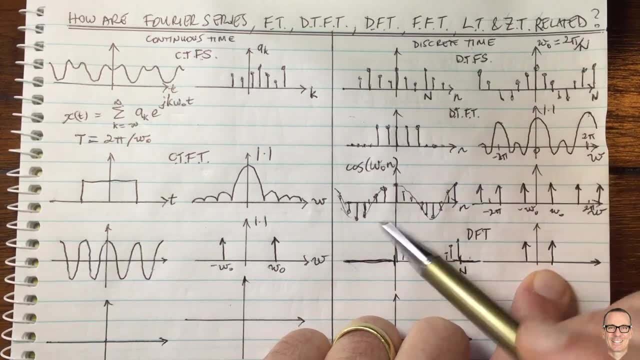 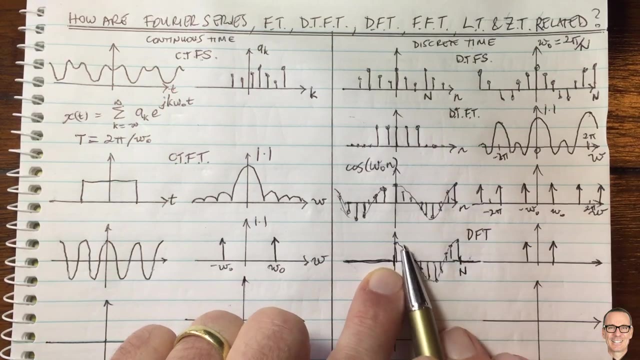 for an infinite amount of time. and so the Fourier, the discrete Fourier transform, will give you exactly the same result as the discrete time Fourier transform, assuming for the periodic signal. so if this signal here were to be, if this was a cause that you have sampled, then the DFT 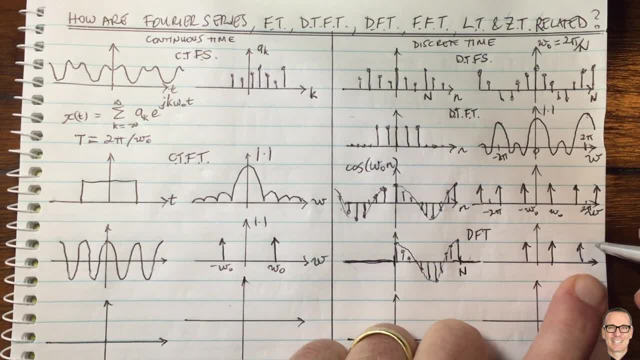 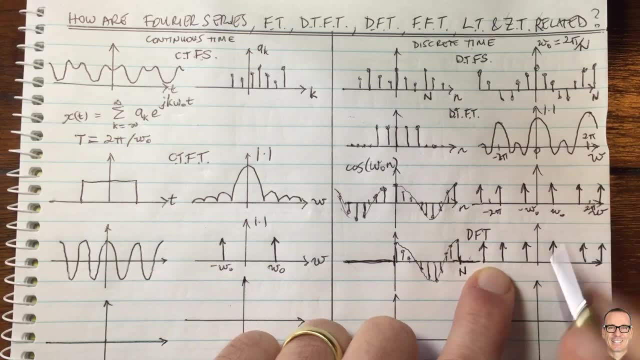 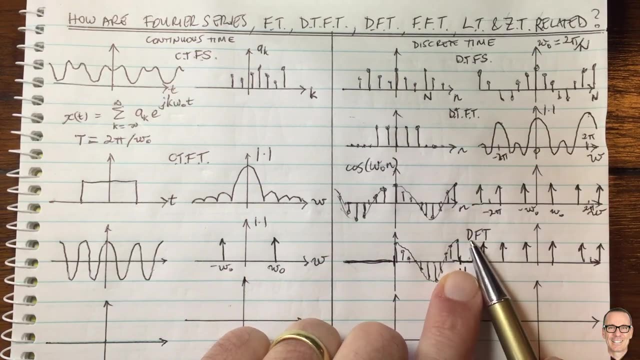 process assumes it goes forever. so you'll get, it will give you and you can do this in MATLAB or or other Python and so on programming languages and you'll see that you given back an exact version of the discrete time Fourier transform when you do the discrete Fourier. 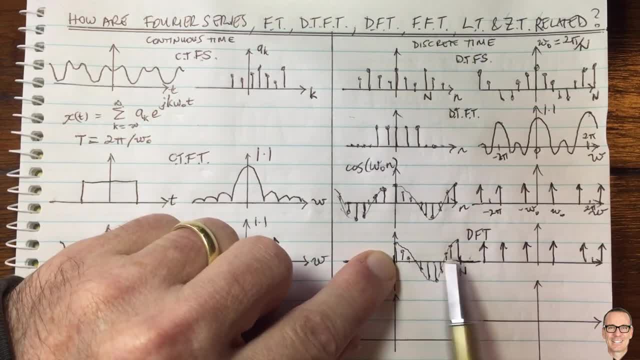 transform now. you can then see what happens. this is the case if you have sampled over an exact period. if I had taken less samples than a full period, then you wouldn't have a waveform, which would be exactly the same as cause, because you would have a shorter waveform. 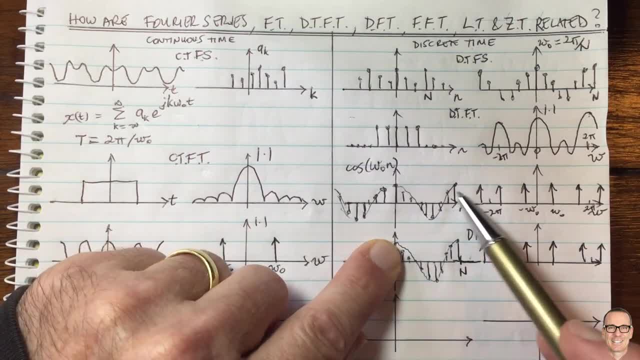 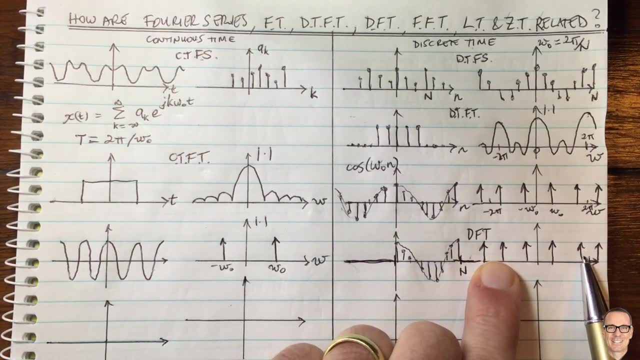 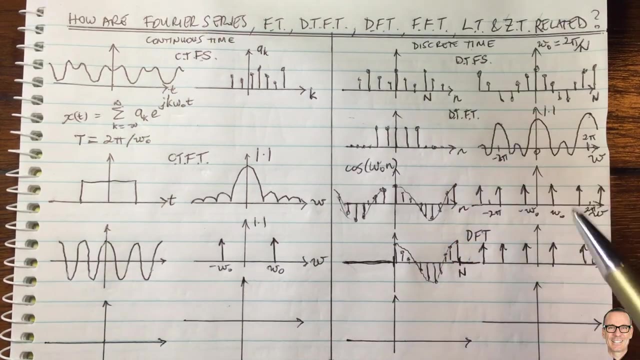 which then would not repeat periodically to form a cause because it would have discontinuities at the ends and then you would not get exactly matching into in the frequency domain. and again, there's a video on that on the channel about the DFT. okay, so what is the FFT? well, the FFT is: 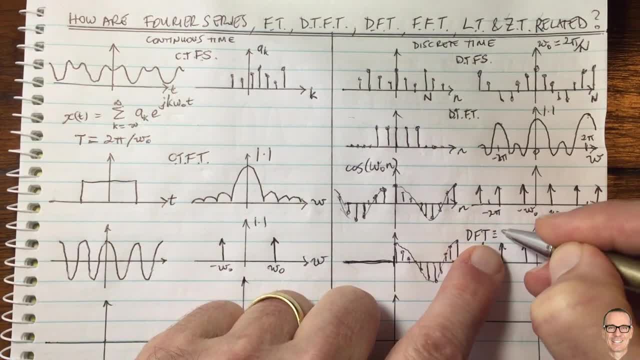 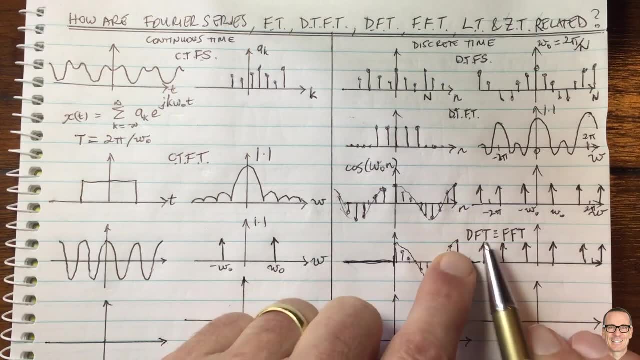 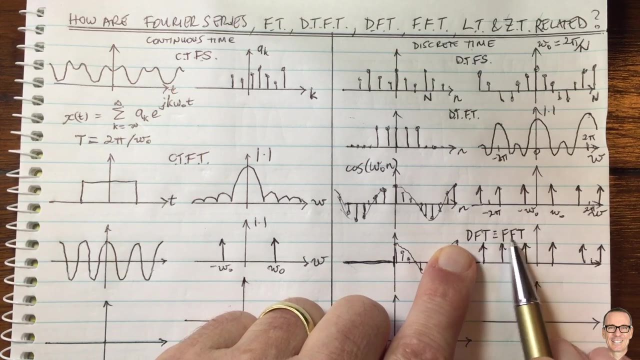 exactly the same as the DFT. it's just a clever way of implementing the DFT in a fast way, of fast using less calculations than the Fourier transform. so if you have a full period of time Fourier transform, you can then see that the FFT is the same as the discrete Fourier transform. it's just a more. 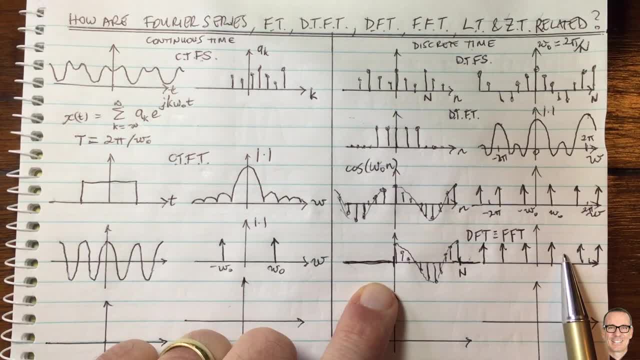 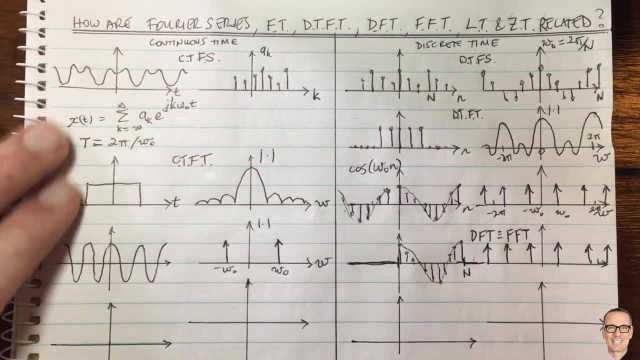 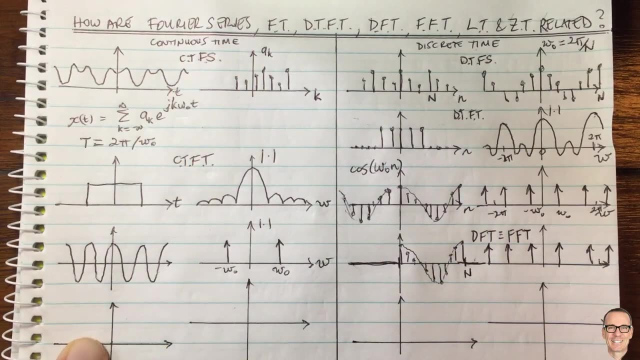 efficient implementation. so you get the same relationship there. okay, and the last two transforms of the Laplace transform and the Z transform, and in the Laplace transform. how does that relate? well, the Laplace transform is in continuous time, the Z transform is in discrete time. so let's look at those two now. so we said before that the Fourier transform applies for 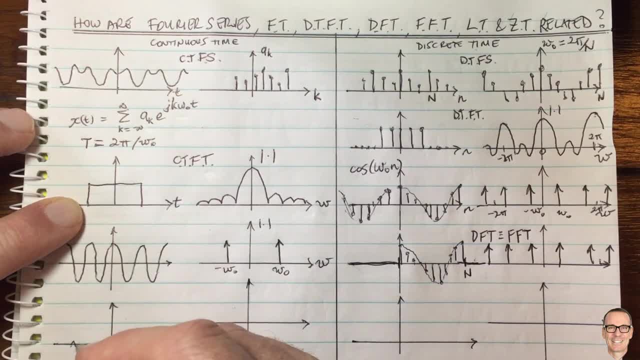 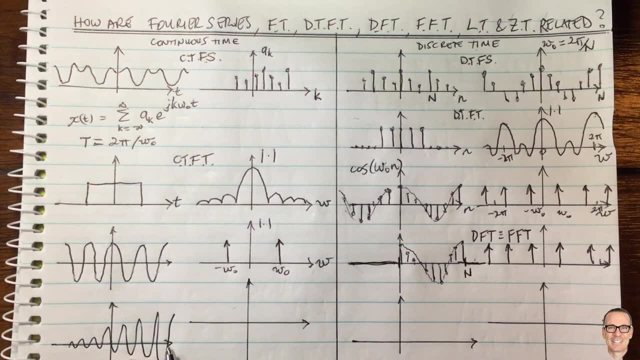 signals which have full DFT, and the Laplace transform applies for signals which have full DFT- finite energy. so what do you do if you had a signal like this, which is continue oscillating and continuing to increase? so this is like, for example. one example is positive feedback in a 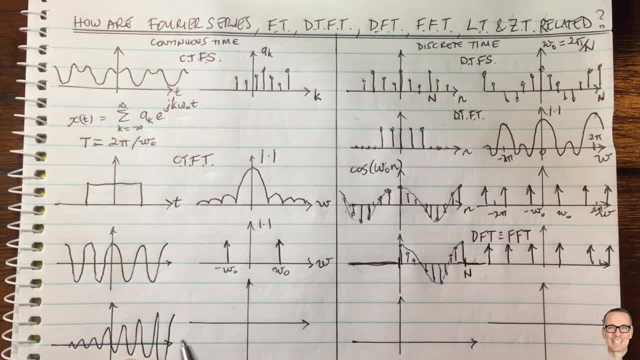 microphone system where the signal keeps increasing in its amplitude as time goes on. well, this signal, if it keeps going like that forever, it will not have finite energy. so in this case, instead of doing the Fourier transform, in this case we generalize and we, instead of having J Omega in the formulas which I haven't shown the formulas here, but you can look them up. 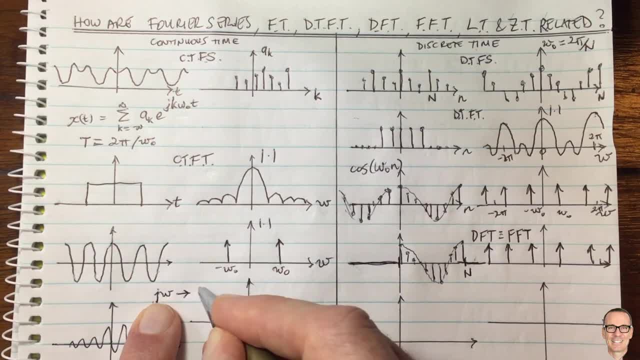 instead of having J Omega in the formula, we replace that by another variable, s, which simply equals Sigma plus J Omega. so it's almost the same as the Fourier transform, it's just that there's an extra component, a real component, in which you're replacing it by and again. there's a video on this. 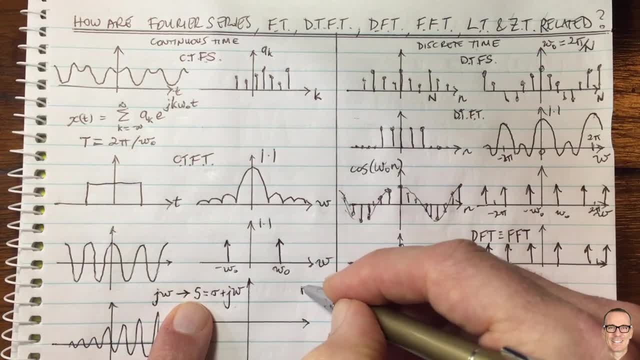 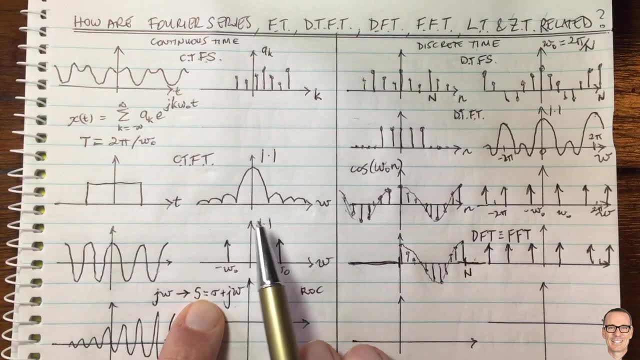 that explains the region of convergence and so much more about that in just a moment. so let's go over to Q1 and Q2 and we go over to Q3 and Q4 and I'm going to show you a real example of the Chelsea transformation and you can look at a very little bit of that: the false and flat. 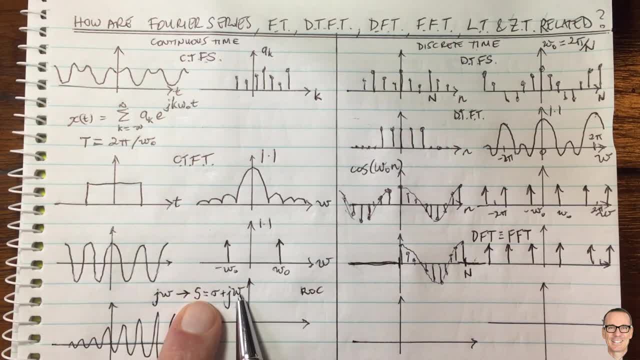 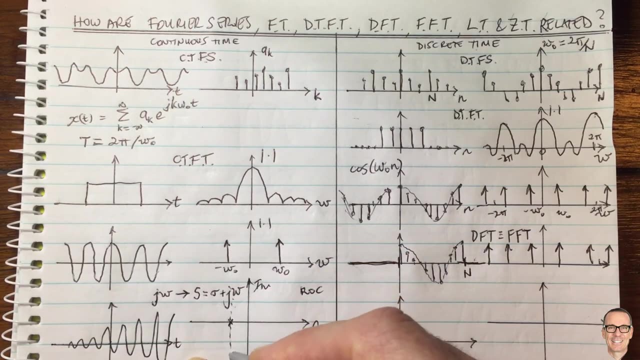 involved with the jelly-shaped and so normally we say: this is the real and imaginary, and your you've probably seen things where there's a vertical, there's poles and zeros and a vertical line from the poles and you might have seen a cross-hatched area and you're probably having a reality where you're seeing this. square shape, which is a vertical shape that turns out to be a straight shape from one to one and you're not going to have a clear picture of the square shape. and then you have a change in the area and you might have seen this. there's a little bit of an pass through, just a little bit of a straight line to the 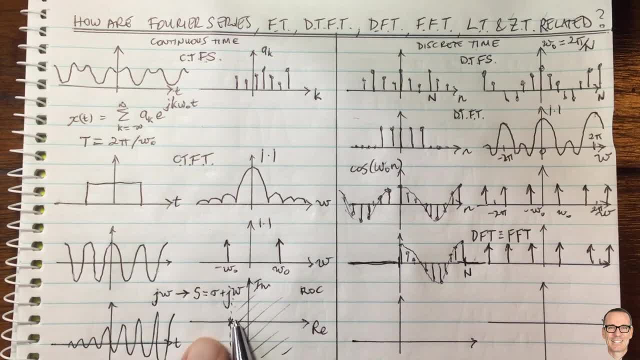 which is the region of convergence. what that means is it's the, the area, the region of s values, which you can see. sigma values are bigger than this. number here, for example, would give you that whole area to the right. so it's its values of sigma for which the transform converges, for which you can 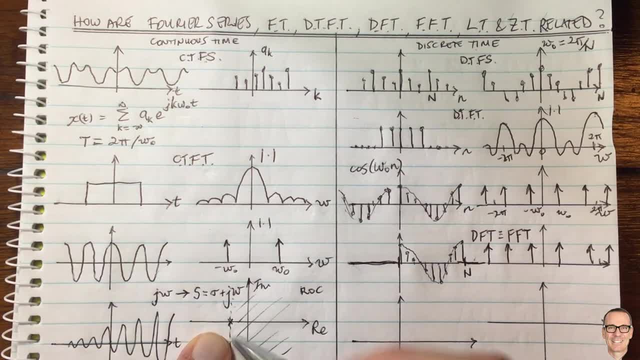 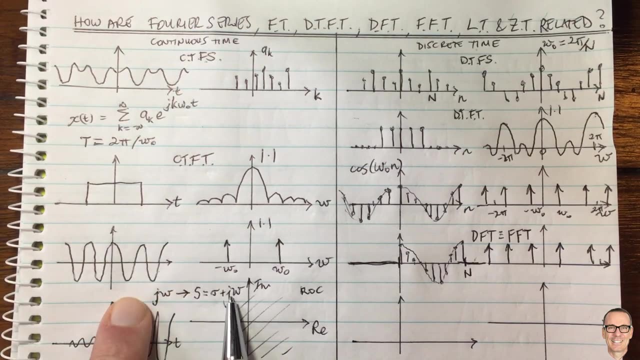 evaluate the integral and it turns out that if you, if it includes, if this region of convergence includes the vertical axis, when sigma equals zero, then you do in fact have the Fourier transform. so you can see here, if sigma equals zero, then you would exactly have exactly the same as the 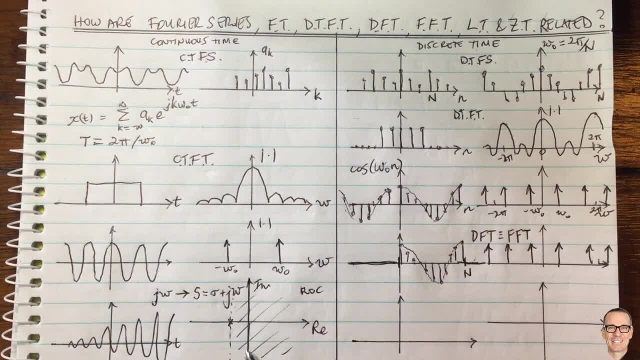 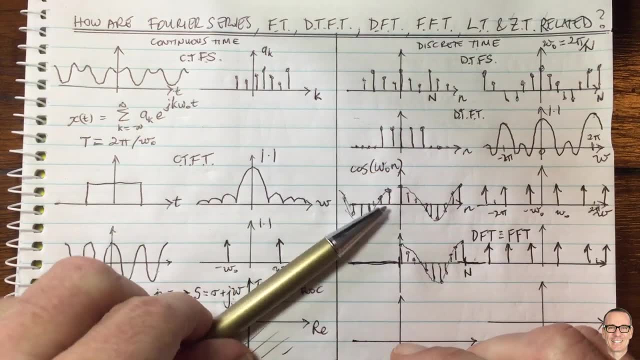 Fourier transform and that would be looking along this line here. so if we took that line- this is where this gets greater here and this gets left- if we took this line and we rotated it around for sigma equals zero, then we would have the Fourier transform. so I think of the Fourier 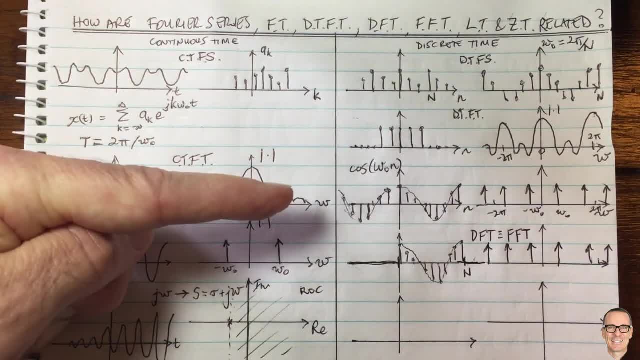 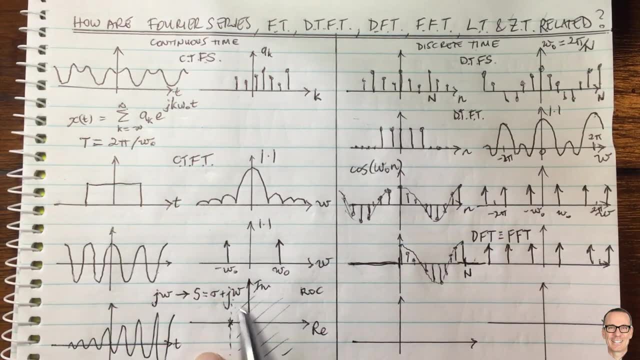 transform that we've drawn in this. you line here. if i flip it up so it's vertical and then shift it around like this, then it lives above that line there and the other values. for other values of sigma, you will have other shapes and there will be a smooth function. and again, for more insights on this, there's a video on the channel. 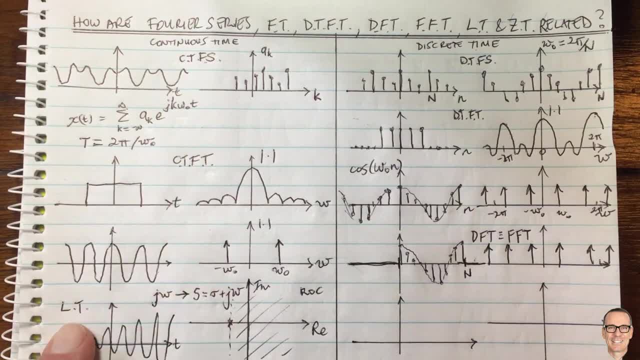 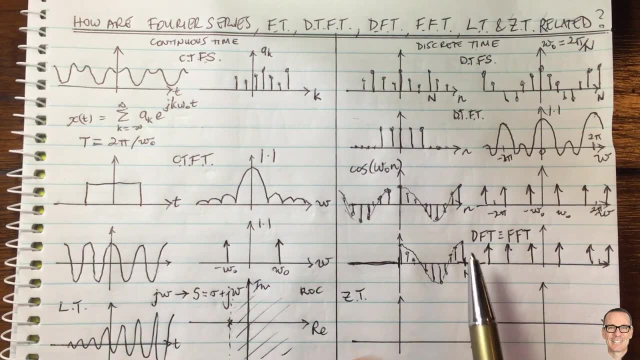 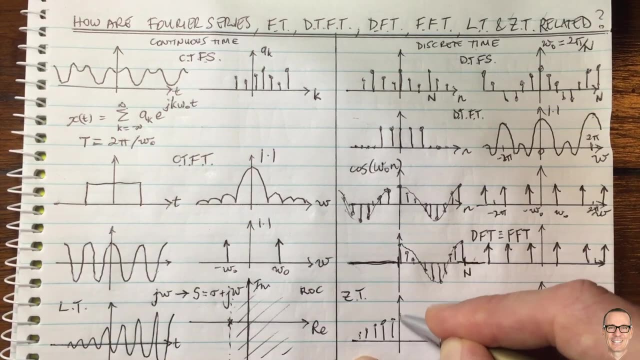 and so the final one is: so this is the laplace transform, and so the final one is the z transform. okay, and the z transform is equivalent to the laplace transform, but just for discrete time signals. so if we had a signal that was increasing as time went on or as the samples went on, 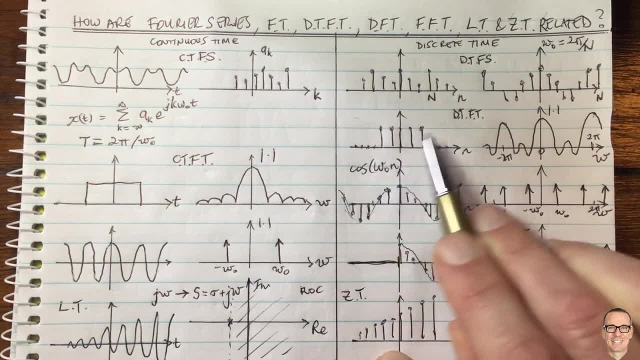 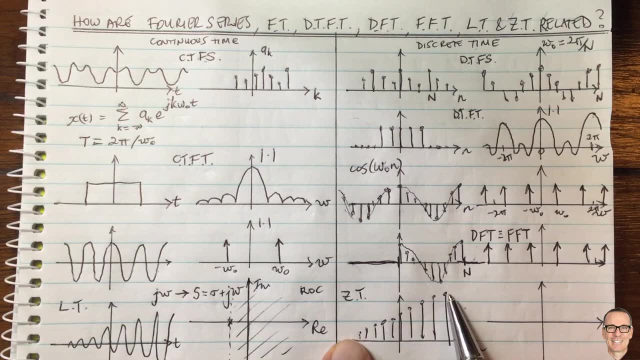 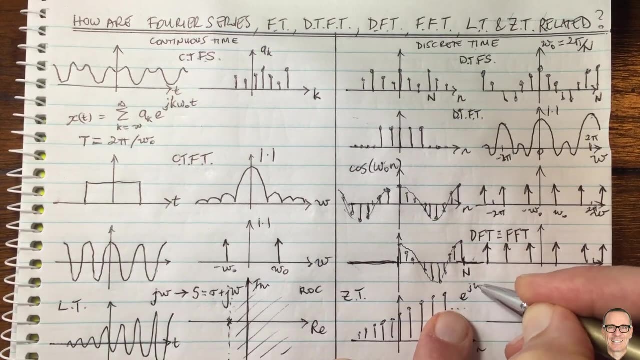 it's not a finite signal, it's a signal that goes forever. so, like this discrete time signal up here, then if this signal here- this is this- does not have finite energy. so again, as with laplace, but in discrete time, we can replace and again you can see more details. 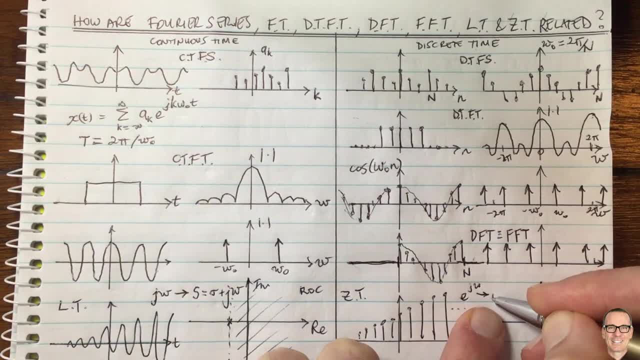 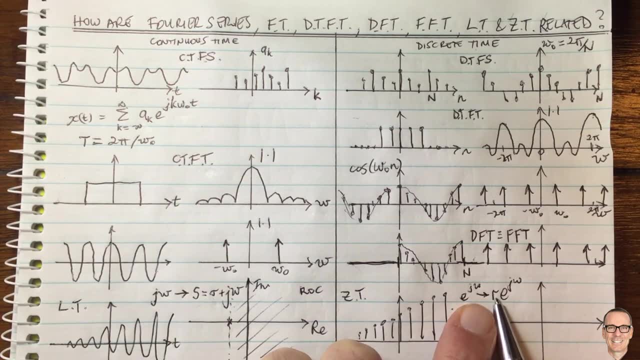 on this. but we can replace the e to the j omega by an r fis Geechee plus two times the z transform r times e to the j omega. so again we're putting a real value into, or we're putting an amplitude here into our pot. this has been polar coordinates, where we put a real value in over here and i 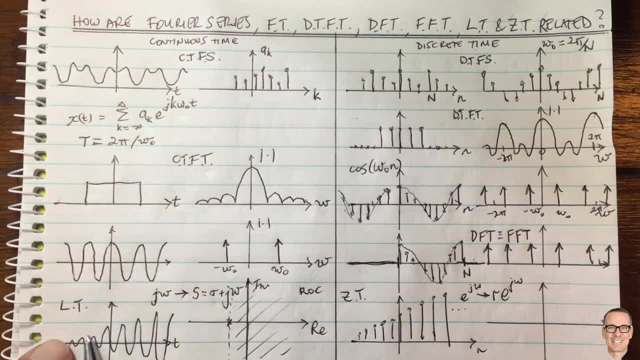 should just go back and say: the real value here dampens this expansion, so it ends up by multiplying this. the effect is to multiply this function here by an exponential of the reverse slope so that in the overall signal resulting from doing that doesn't grow and is finite. and again you can. 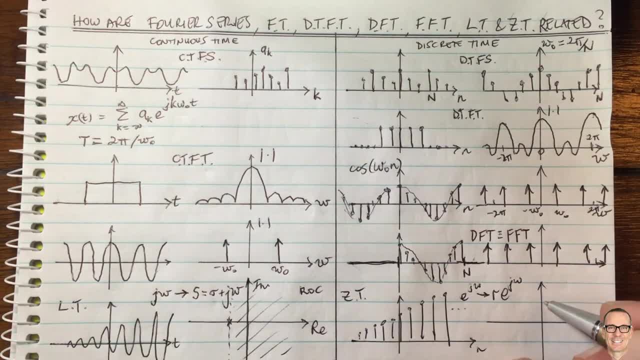 see more on the video about the region of convergence for the laplace transform. in the case of the z transform, it's in polar coordinates and so you'll see that there are circles, there's a unit circle in and and you, you, you get other, another circle, let's say inside the unit circle. 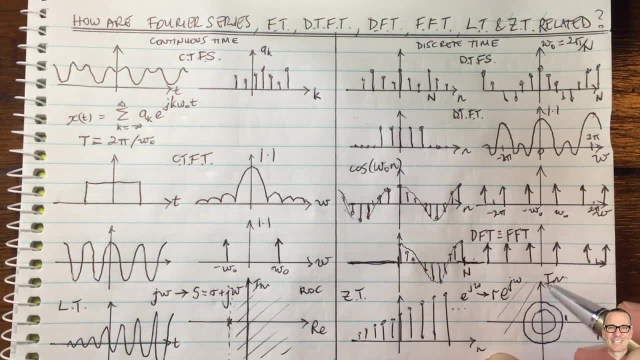 so let's say that was one. and so again you get a region of convergence which goes from the, where the poles are, and outside that. and so again, for all these values that are in the shaded region, you would get a convergence of your z transform. and so again, when you see